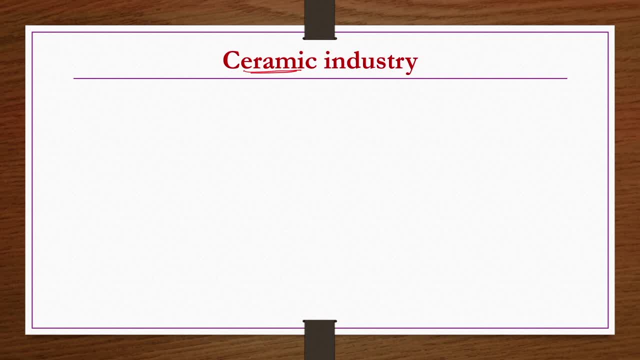 waste or potteries, etc. So because of that reason, traditional name of ceramic industries is also clay products. Not only clay products, it is also known as silicate industries because most of the clays are having one or other kind of silicates. So that is variety of 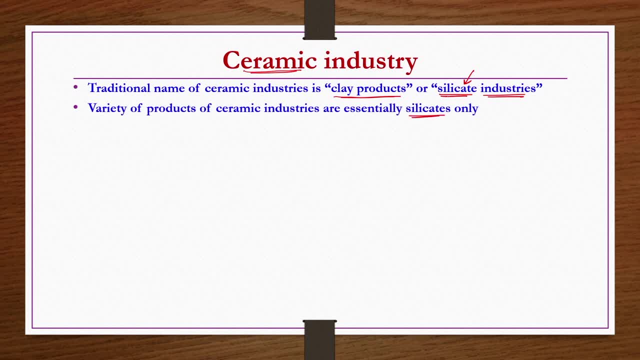 products of ceramic industries are essentially silicates. only Because of that reason, the ceramic industry was known as a silicate industries in earlier days, traditionally. However, nowadays, so many varieties of products of ceramic industries are also known as silicate industries. So 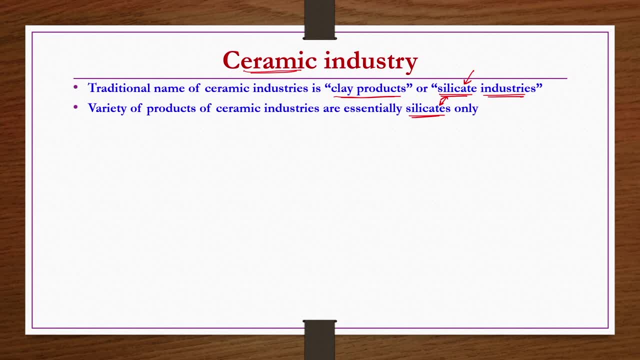 we are going to discuss about ceramic industries, So let us get started. Many varieties of products have been developed based on the consumer needs, etc. So because of that, one calling ceramic industry silicate industry in today's context is not appropriate. 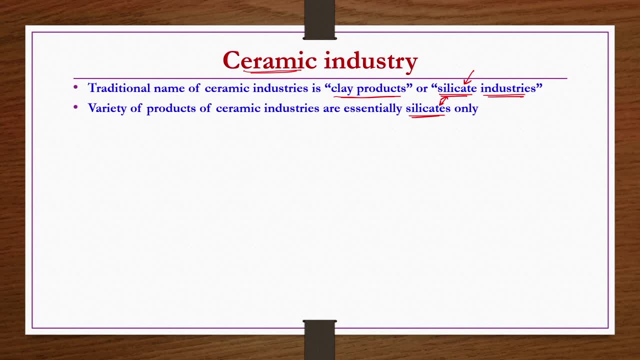 because there are some kind of ceramic products which are produced with some basic knowledge or basic information input, not only from the knowledge point of view but also from the material point of view. Some inputs are there from the metallurgical industry as well, So calling them only silicate industry is not appropriate in the present-day. 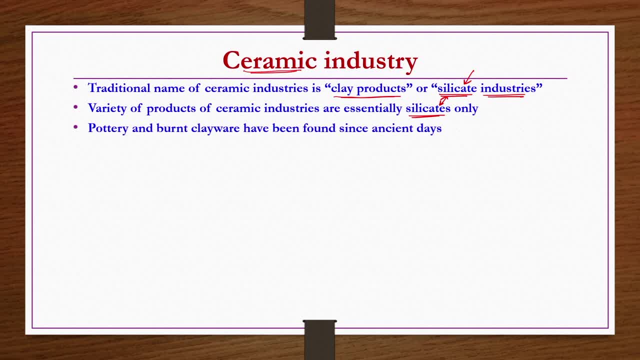 content. Some of the ancient days examples of ceramic industry products are pottery and then burnt clayware etc. But nowadays demand for superior materials have led to broader spectrum of products. Earlier you have only some kind of pottery or clayware only were being produced. 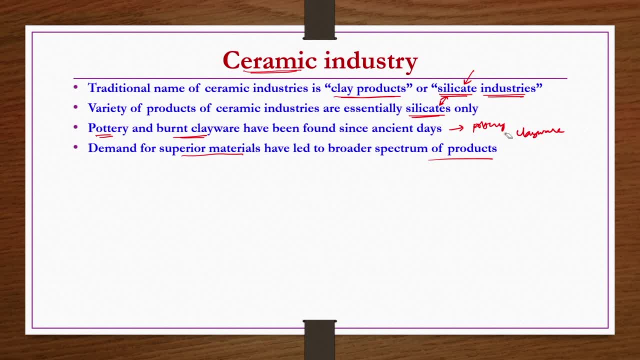 in ceramic industries. But nowadays, what happened? so many demands have come for different types of products, like you know, some kind of semiconductor chips also. there also, it is required to have, you know, specified design and then product requirement, which are produced not only from the products, not only from the raw materials of the ceramic industry, but also from metallurgical. 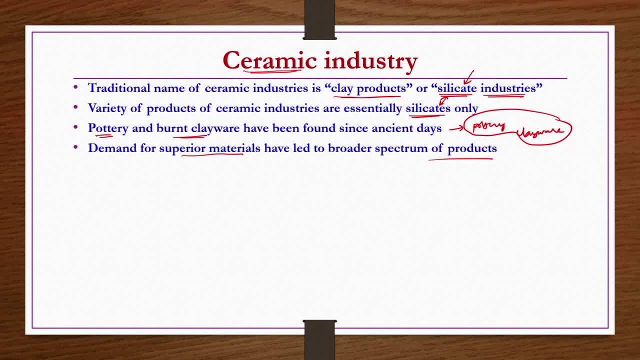 industry also. For example, like many people, in place of their broken teeth they used to have a silver crowned or gold crowned teeth, etc. they may be implanted right. So there you know, a kind of a cross fertilization of ceramic industry with metallurgical industry. 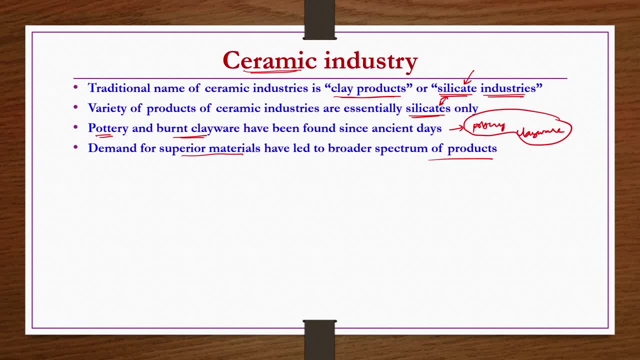 is done. Similarly for several semiconductor chips. also, some kind of combination of ceramic industry knowledge and then metallurgy knowledge is required, okay, So because of such kind of demand for superior materials or different types of material, the spectrum of products of ceramic industries has become very broader these days. 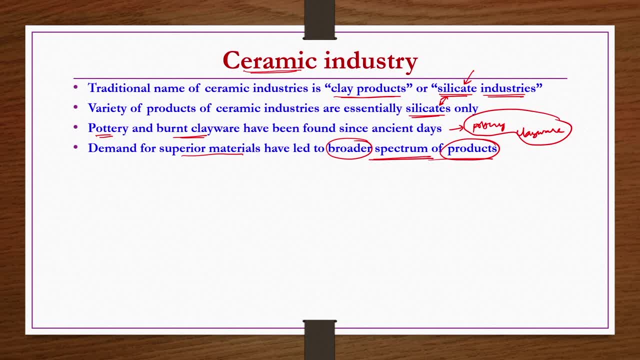 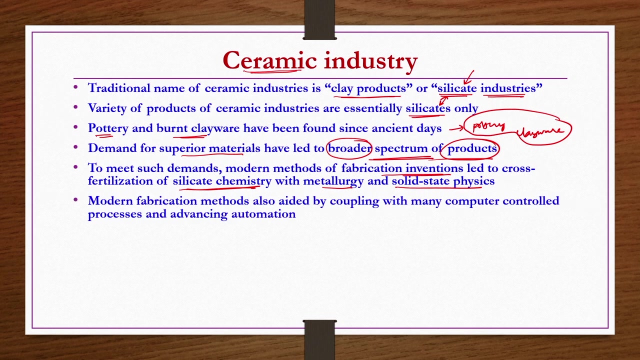 So when you have a broader spectrum of products, then obviously you need to have, you know- much more input to get such kind of products. So in order to meet such demands, modern methods of fabrication, inventions have led to cross fertilization of silicate industry with metallurgy and solid state physics- okay. 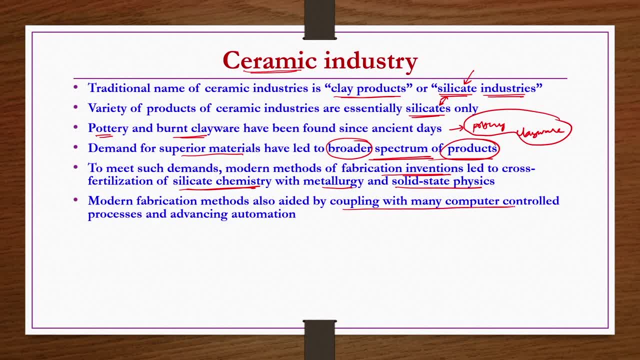 Modern fabrication methods, also aided by coupling with many computer control processes And advancing automations. because sometimes when you prepare such kind of semiconductor chips etc, and then gold crowned teeth etc. you know you need to control the process conditions very specifically of required temperature within plus or minus 5 degrees centigrade. 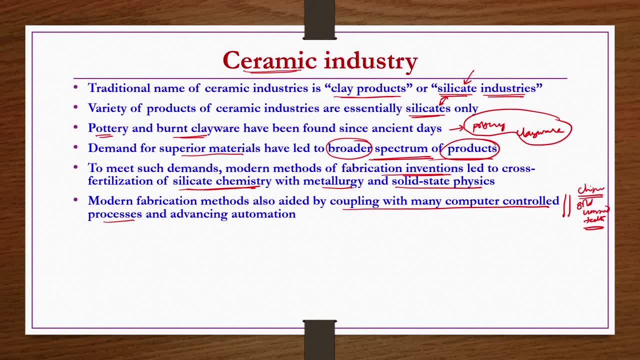 especially when the operating temperature is very high, in the range of 900 or more than 900, or 1000 degrees centigrade, etc. you know, Controlling temperature, Controlling temperature within small range of error of plus or minus 5 percent degree. 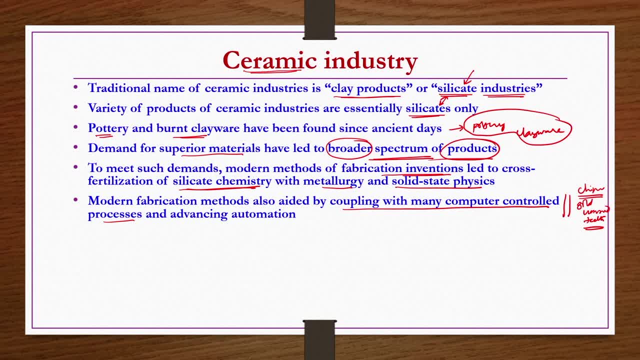 centigrade is very difficult when the range of operating temperature is very high, like you know: 1000 degree centigrade, 1200 degree centigrade, something like that. So for that it is very essential to have computer control processes and then advancing automation. 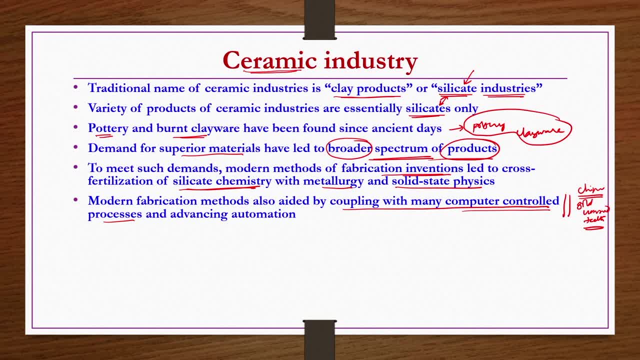 technology you know are very much essential for the growth of the industry. Not only from, you know, basic raw materials of ceramic industry And then with some inputs from the metallurgical industry, variety of ceramic products are produced, but also from waste also, different types of ceramic products are in general developed. 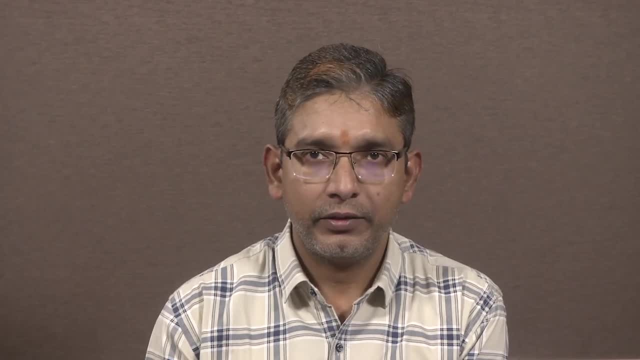 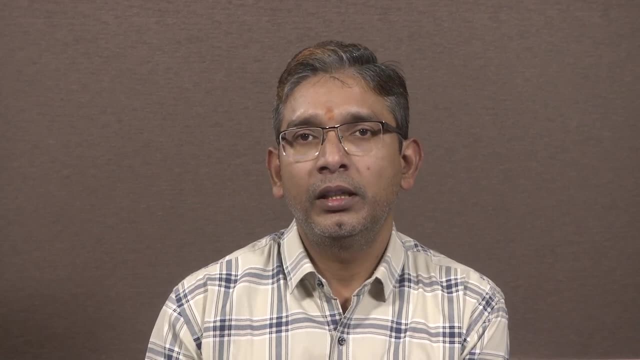 Something like. you know some inorganic waste like fly ash from the power plants. You know that may be fly ash. usually- you know mostly- is a waste product. It is not being utilized for any other purpose. so that is being utilized by the ceramic industry to make different types of bricks. you know. 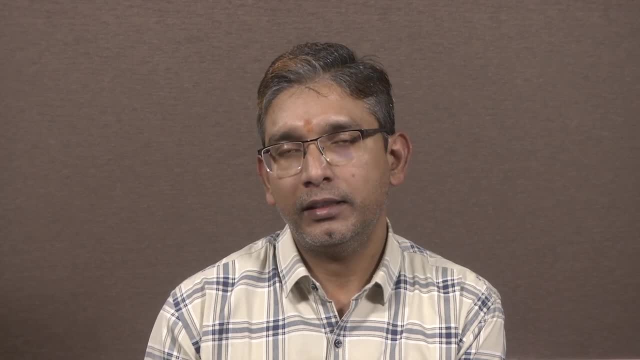 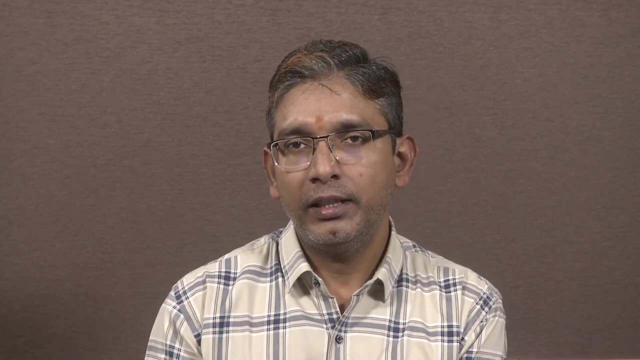 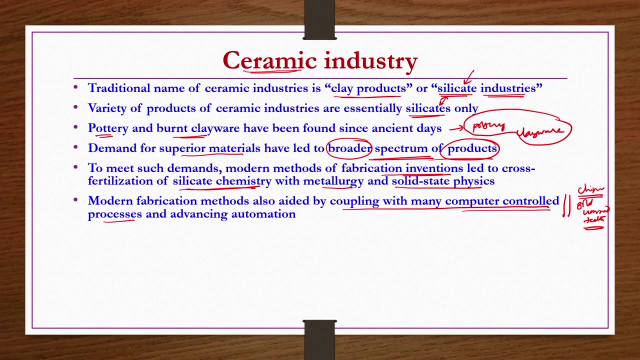 Okay, Similarly mine tailings, etc. they are also a kind of wastage project from the prospective of the mine industries, right? So those mine tailings also utilized to get or prepare some kind of bricks or ceramic products. Likewise, you know metal slags in metallurgical industries after getting the refined product. 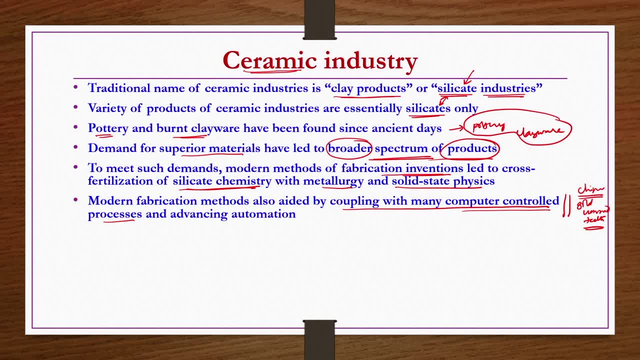 of required nature, required characteristics, a lot amount of metal slag is produced. There may be important ingredients in those metal slags, but recovering them may not be economically feasible, right? So because of that reason it is better to utilize them for some other application. 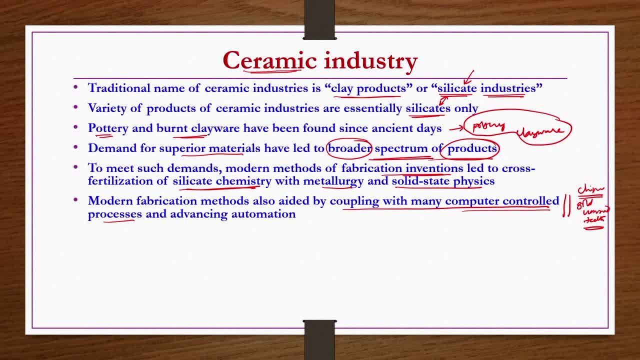 So such kind of metal slags are also used for a brick making kind of thing, which can be done by ceramic industry principles. So thus, as explained, several types of bricks can be made from different types of inorganic waste. And then, what are the such inorganic waste? 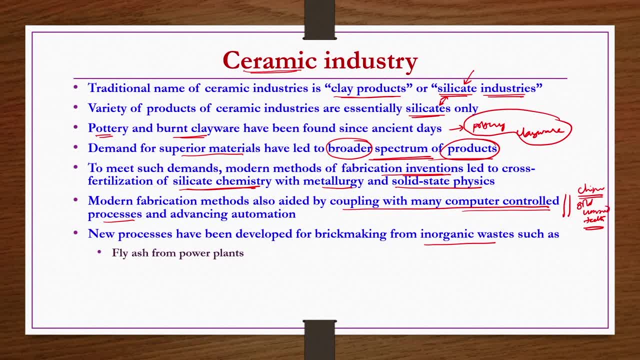 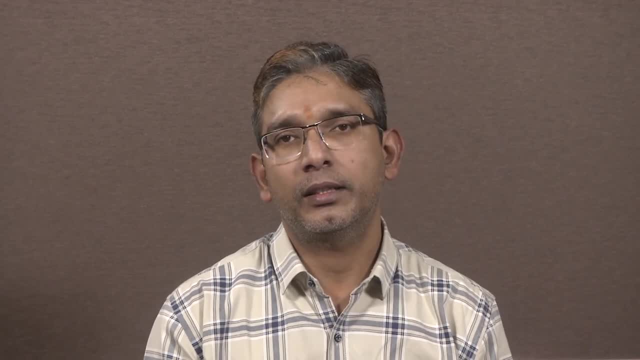 Which can be utilized for making bricks, fly ash from power plants, foundry sand, mine tailings and then furnace slag and a large variety of other materials as well. Now from the product point of view. if you wish to have a product from a ceramic industry, 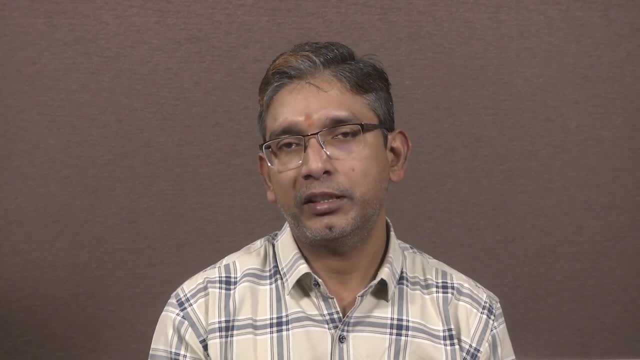 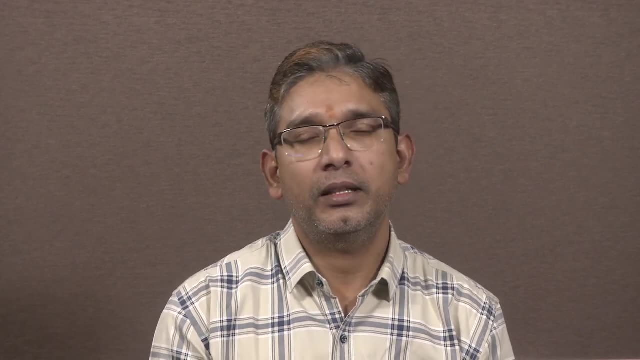 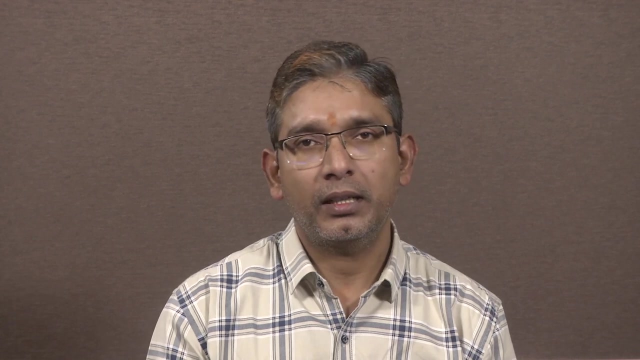 what kind of characteristics you supposed to expect or you may be expecting in general, So especially, you know, from the applications point of view. either in plant applications or in household applications, or societal applications etc. you first see, like that material must be mechanically stable, that must be chemically stable, that must be thermally stable, such 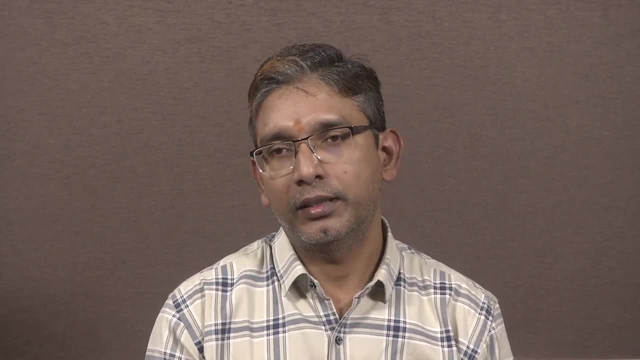 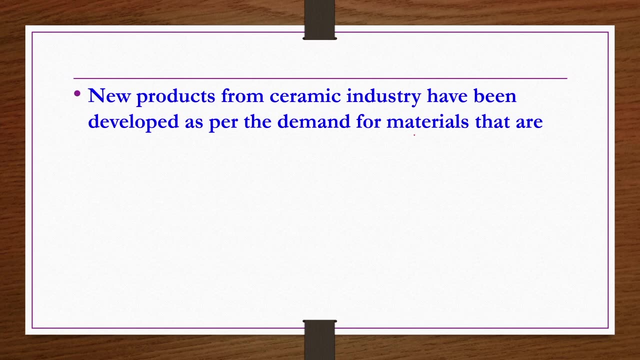 kind of characteristics you see. So those characteristics we are seeing now, New products from ceramic industry have been developed as per demand for materials. Those materials should have following characteristics: thermally stable materials. you can say thermally stable. They can withstand higher temperatures, higher temperatures of several hundred degree centigrade. 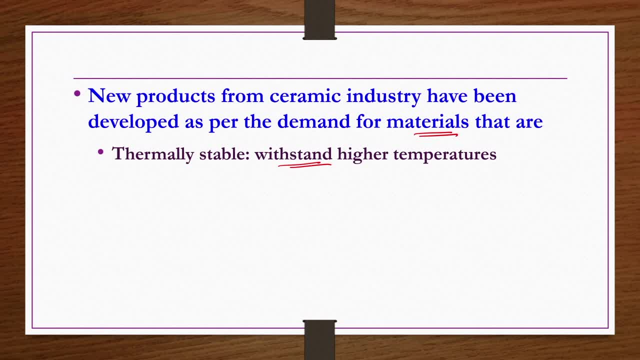 or even sometimes more than 1000 degree centigrade. also Let us say furnaces, like from the chemical industry point of view or application industry point of view. these furnaces are made up of several types of refractories, right, So we have seen some of the refractories are used for making glass making, etc. in one of 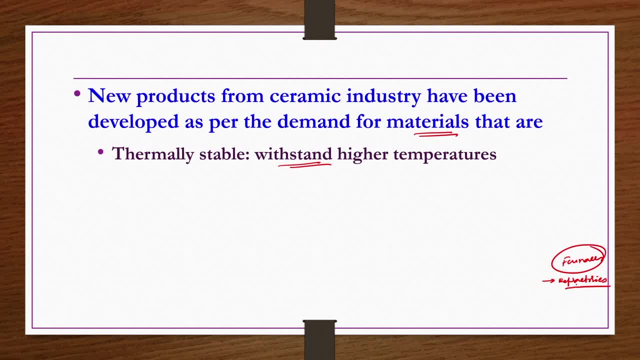 the previous week lectures, right? So now what we have seen. So the operating temperature in those furnaces is very high, order of 1200 to 1400 degree centigrade, something like that, right? So the raw materials are fed into the furnace and then furnace is supplied energy so that 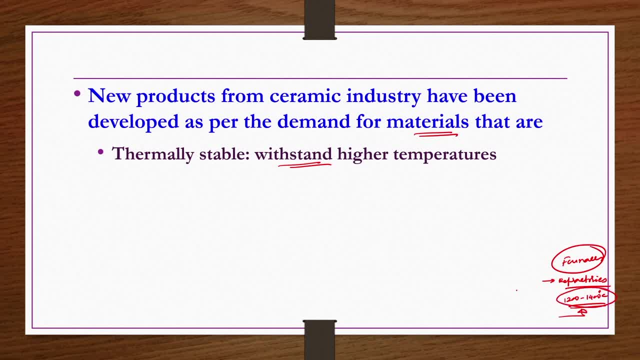 to raise the temperature to, you know, required temperature of 1200 or 1400 degree centigrade, something like that. So at this temperature definitely there would be reactions amongst the materials that have been fed to the furnace right. 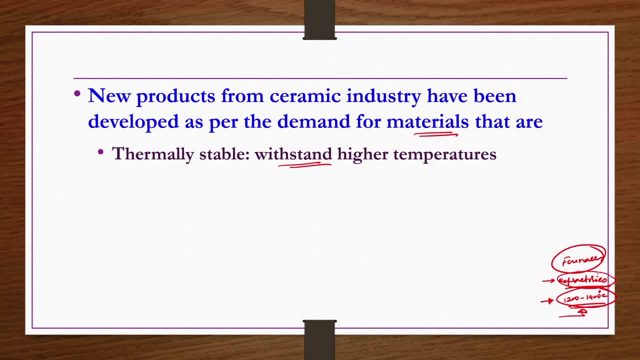 So now let us see what we have seen. So the operating temperature in those furnaces is very high. So now the refractories that are being used to make this furnace. they should be chemically stable as well as the thermally stable. 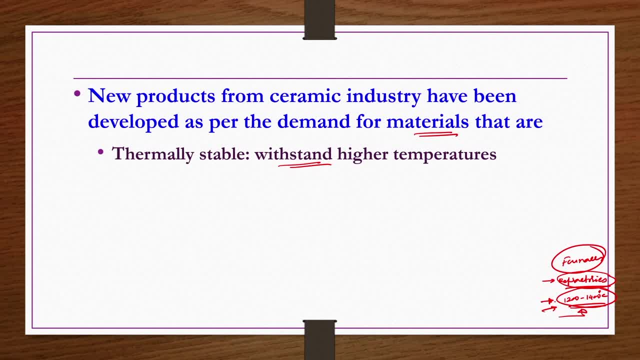 Thermally they should be stable up to this temperature or even beyond that one. And then, what are the products are forming? chemical products are forming. What are the input chemical reactants given to those furnaces at such high temperature? So these refractories should be chemically stable to those chemical nature of the components. 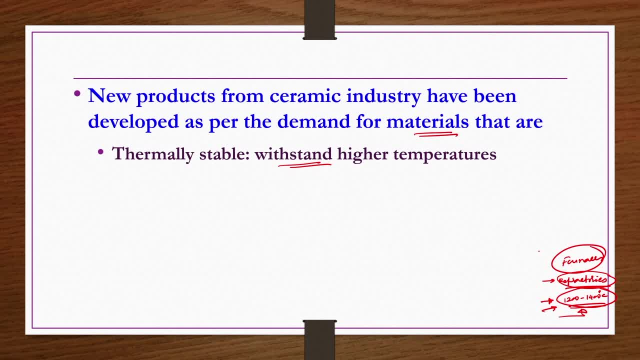 as well. So that is also required. So this is from the chemical industry point of view. Okay, So this is from the chemical industry point of view. right, If you have a sewage, you know sludge, etc. they are allowed to flow through certain kind. 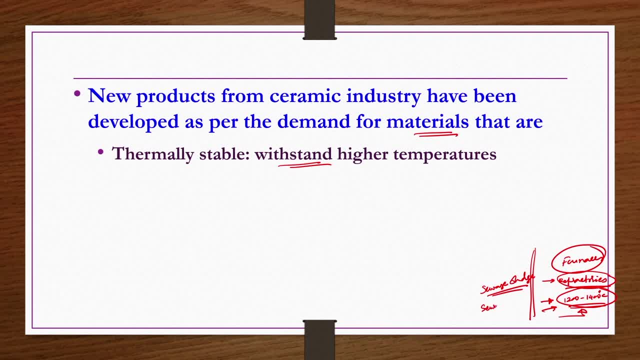 of enclosed area where you need sewage tiles, etc. So these sludges etc are very acidic actually in general- though the temperature may not be very high in such conditions- but they are very acidic, right? So then you know when the material or sludge passes through such enclosed area, which is 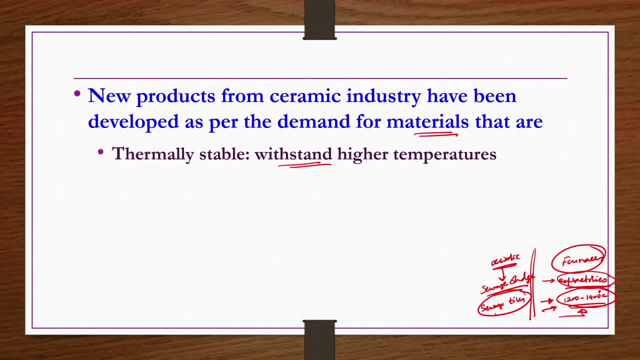 you know, covered with the sewage. So then these sewage tiles should be, you know, chemically stable against those kind of those acidic sludges etc. So chemical stability is also required. So, like that, if you keep on saying that mechanical stability is also very much essential, right? 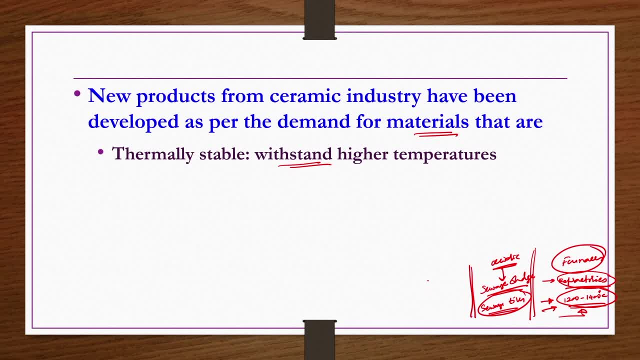 You know floor tiles etc. you in general have. And then you know sometimes you know what happens at the household purpose or office hold purpose also. you may be shifting or moving the furniture from one place to the other place and then weight of such furnitures may be very high, in general some hundreds. 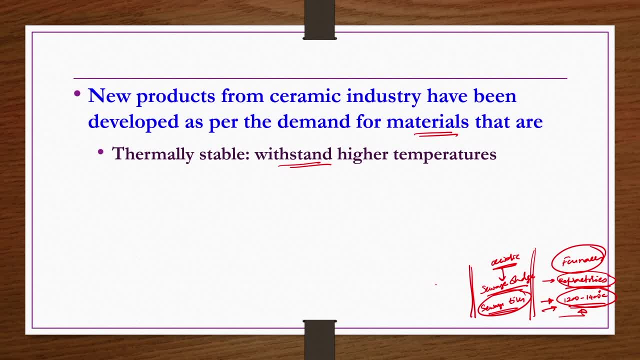 of cages or something like that. So if these tiles, floor tiles etc. are breaking to such mechanical weight itself, so then that is not going to good. So that is the reason you know you need to have a mechanical stability in your product. 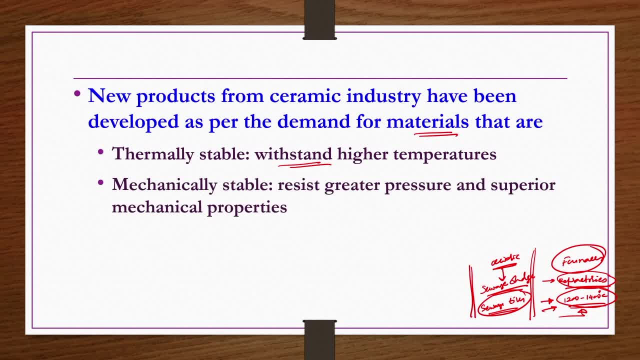 okay. So the second one is mechanical stability, So that product should resist greater pressure and superior mechanical properties. Then chemically stable: They should protect against corrosive chemicals. right, Sometimes you know your product, your ceramic product, should have all these three characteristics. 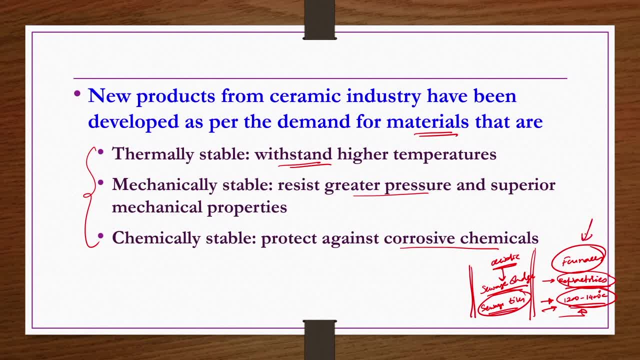 as per requirements. Let us say furnaces made up of refractors, etc. one good example, right? Such kind of examples we have already seen in other classes where you know glass making and then cement industries, etc. In those cases we have seen- you know so much of, you know- these materials that are. 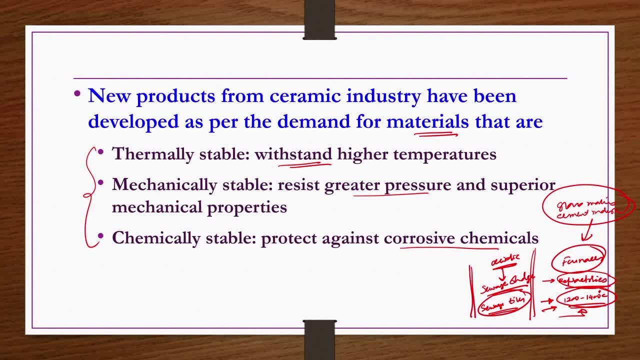 used for the ceramic making. you know they are also there. So you expect to have all these thermal stability, mechanical stability and chemical stability in one single applications. In sometimes in for given applications, you may look at only one particular important characteristic, like you know, thermal stability. other applications you primarily concentrate. 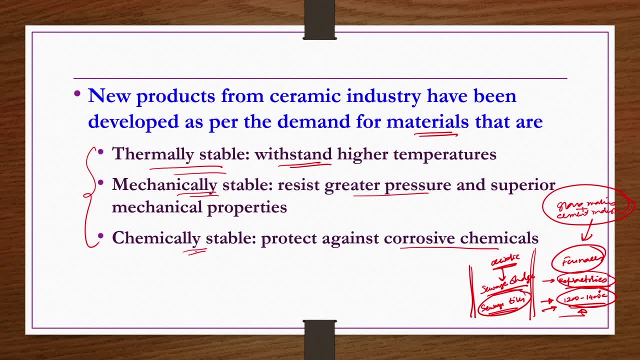 on mechanical stability, other applications. you may concentrate on chemical stability, But sometimes you know there may be cases. Okay, In some applications you may require to have a stability against the thermal applied temperature, mechanical forces and then chemical corrosiveness, etc. all of them together 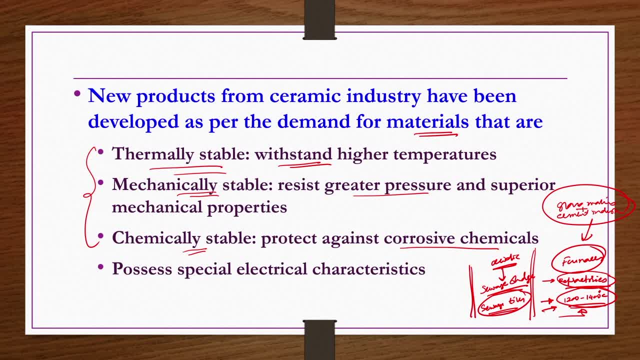 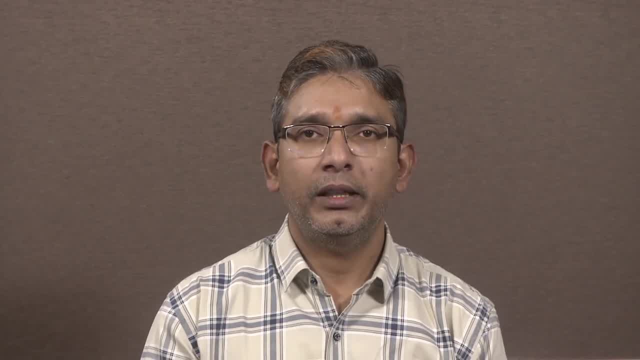 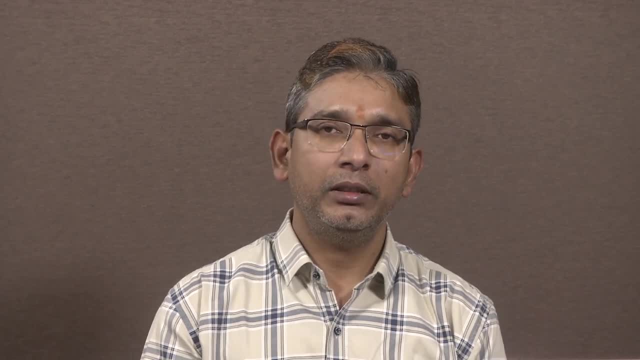 Also possess special electrical characteristics as well. okay, So those are the requirement of ceramic products. You supposed to expect, or you are expected to make a ceramic product which is thermally, mechanically and chemically also stable, right? So now, what could be such kind of products in general? 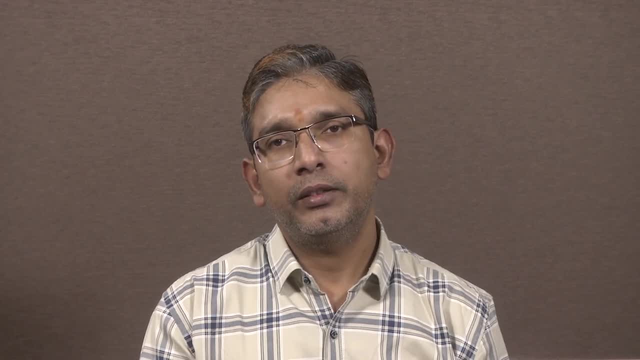 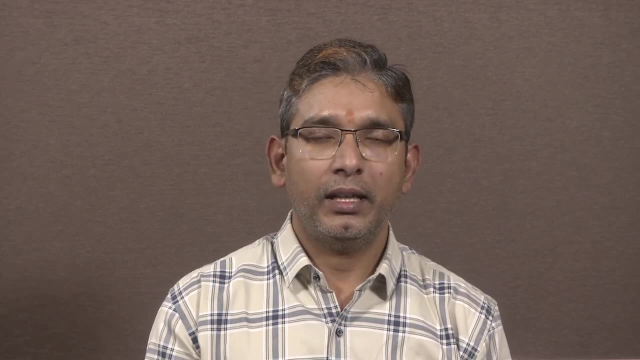 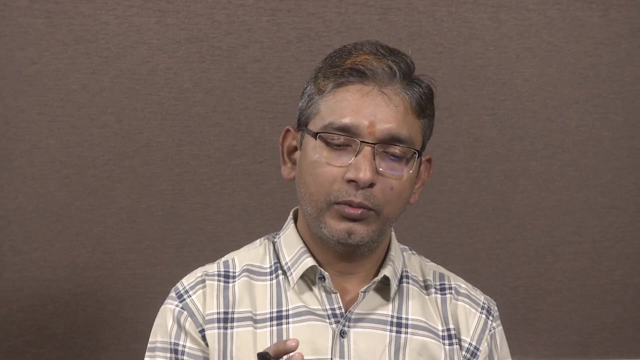 So, if you see, you know range of ceramic industry products is now broader. It is no more very limited in general. So, however, we try to have a classification of different types of ceramic industry products and then see what are they, and then we will be discussing about those kind of ceramic. 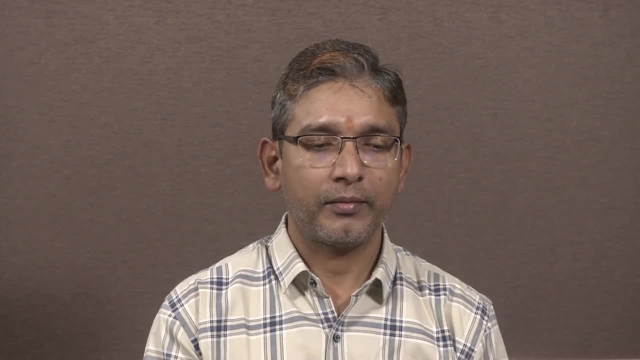 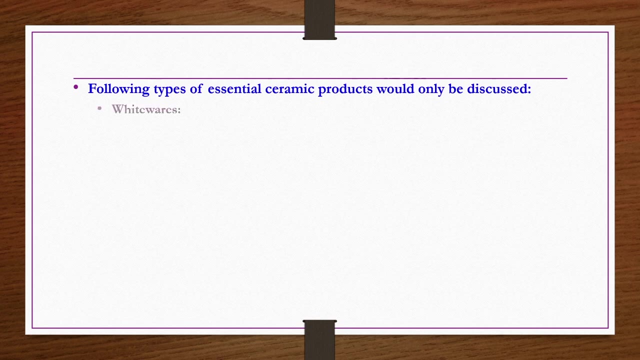 industries products. only in this and in coming lectures Following types of essential ceramic products would only be discussed because of time limitations. okay, So white waste is one type, another one is the structural clay products, another one is the refractories, fourth one is specialized ceramic products and then finally, enamels. 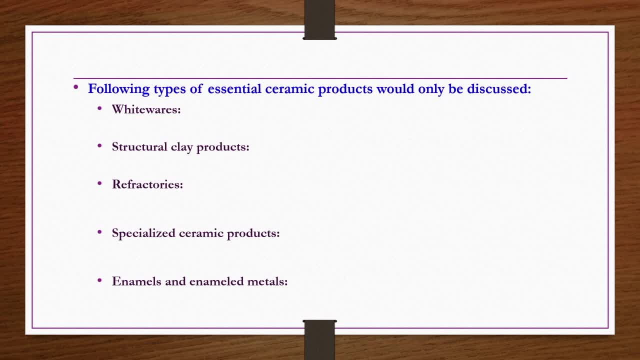 and then enameled metals. These five types of ceramic products we are going to discuss in detail, from their manufacturing, applications and then uses, etc. point of view. we are going to discuss these five types of ceramic products Now. what are the things? 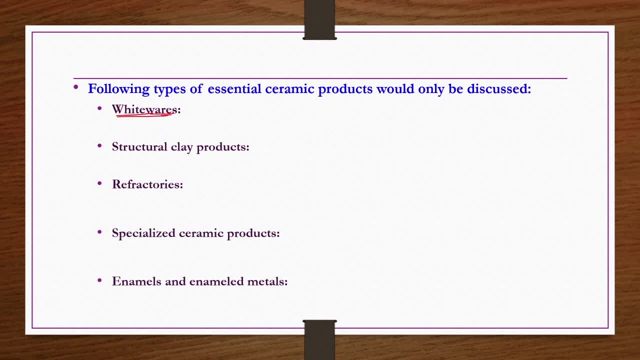 What are the products that are covered under the white waste or what are the ceramic products that comes under white waste? They are nothing but china ware, earthen ware, pottery, stone ware, vitreous ware, etc. By name white ware. why the name is given white waste for them? because mostly their 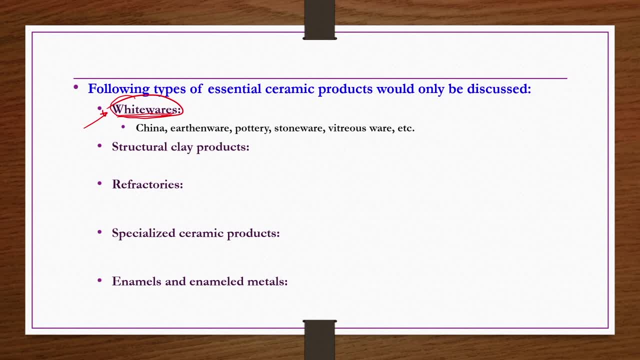 appearance is white in color. There may be some kind of textures and then some designs may also be there of different colors, but primarily these products, you know they are in white in color. So that is the reason That is why they are known as white wares. 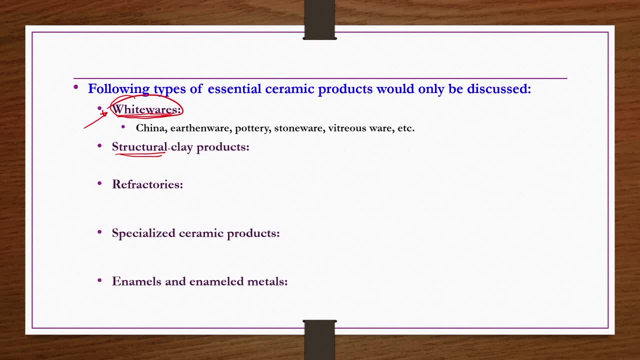 Similarly. second one is the structural clay product. Structural clay products- the name by the structural means the products that are produced by ceramic industry. they are used to make some kind of structures, like you know, some kind of bricks etc. So those things comes under structural clay products category, that is, building brick. 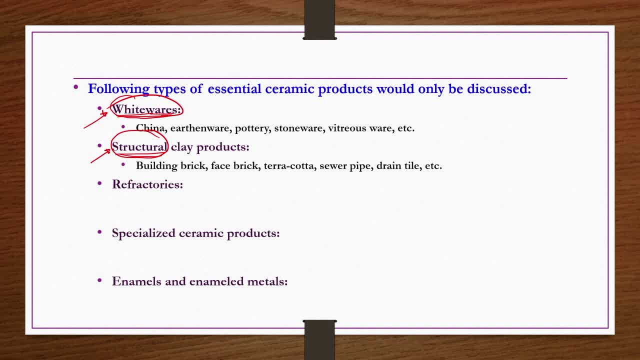 face: brick, terracotta, sewer pipe, drain tiles, etc. Next one is the refractories. Next one is the refractories. Next one is the refractories, which include fire bricks, silica brick, chromite brick magnesite, chromite brick, silicon, carbide brick, zirconia, refractories, and then silicate. 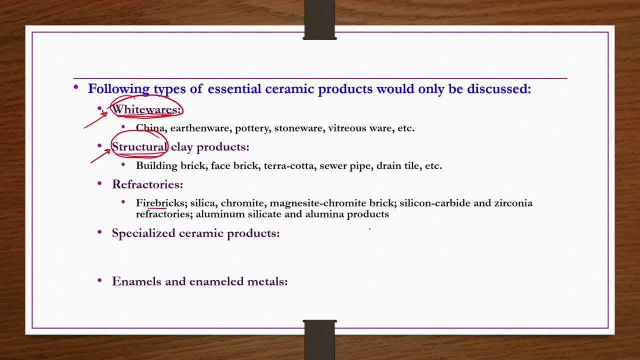 aluminum, silicate, alumina products, etc. all comes under the refractories For the case of specialized ceramic products like gold coated ceramic wafers for semiconductor chips are one of the common application for the specialized ceramic products or it is one of the important product that comes under specialized ceramic products. 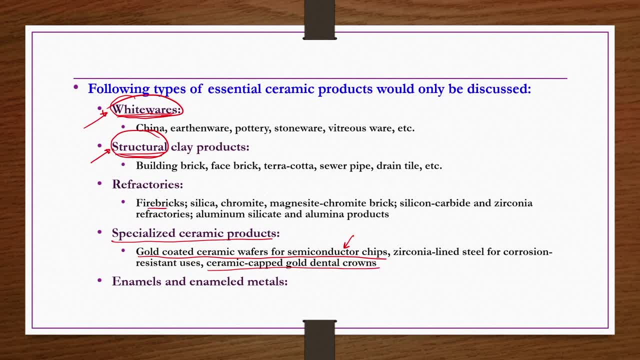 Similarly ceramic capped gold dental crowns and then zirconia lined steel for corrosion resistant uses, etc. all they come under specialized ceramic products. Specialized because they are developed for the specialized applications, like you know semiconductor chips, or you know gold dental crowns, etc. for those purpose special application. 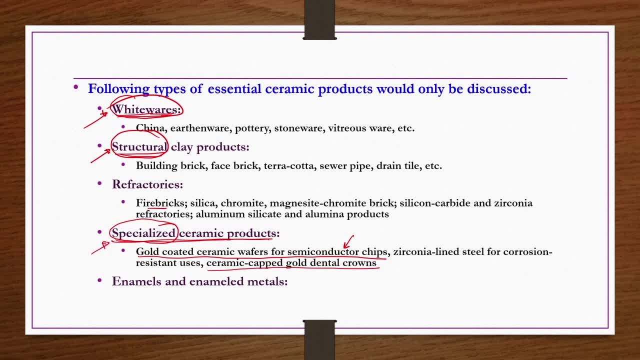 purpose they develop. So that is the reason these products are, you know, called as specialized ceramic products, Thank you. Likewise, under enamels and enamel metals, applications of enamel to gold, silver and copper, etc. used in different types of decorative art, etc. those kind of products comes under. 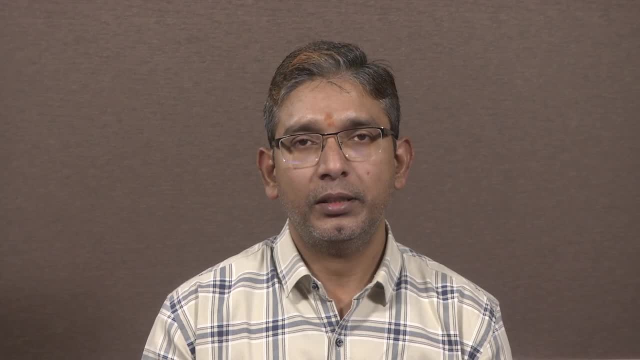 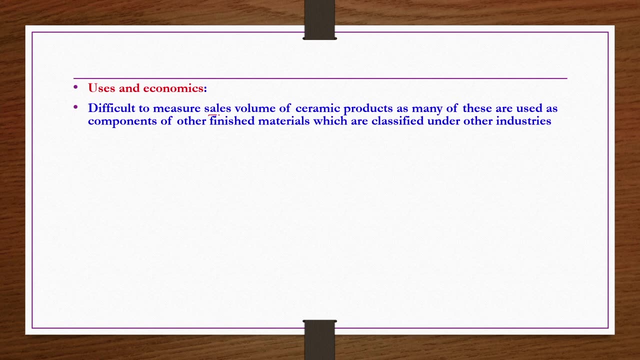 this category. Now we discuss about uses and applications and economics of a ceramic industry. In ceramic industry it is very difficult to measure the sales volume of ceramic products because many of these are used as components of other finished materials Which are classified under other industries. 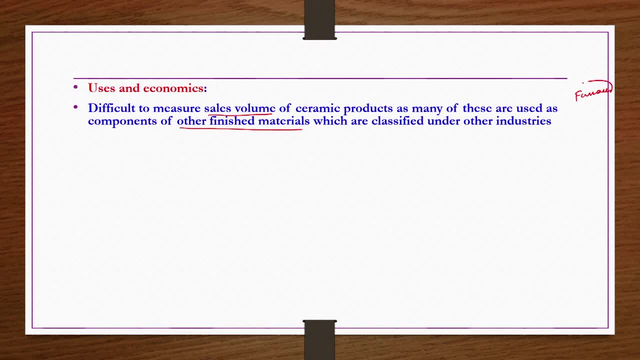 Let us say furnaces, one example. Furnaces, or manufacturing or development of furnaces does not come under ceramic industries. But you know, whatever the refractories are used for making such kind of furnaces, they are produced by the ceramic industry. 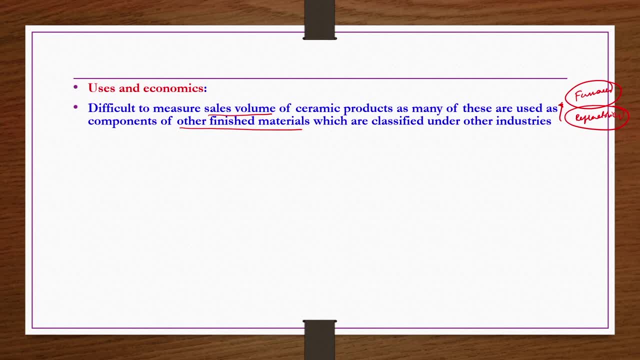 But you know they are utilized for some other industry. that is the reason such kind of many cases are there. You know the products are primarily of ceramic industry, But from the end, use wise. They are in some other industries or for some other purpose. 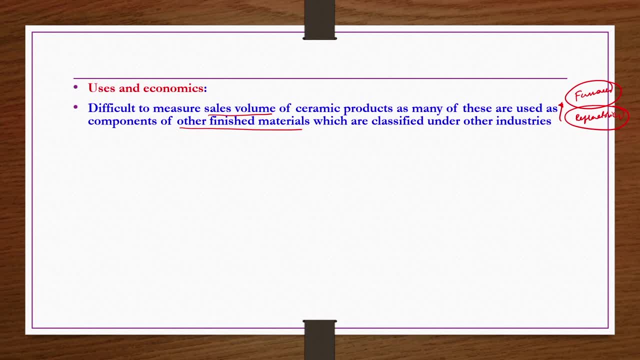 So that is the reason getting or measuring the appropriate sales volume of ceramic products is very difficult. Up to 60 percent of all clay produced- clay not the product clay produced utilized in the manufacture of heavy clay construction products. and then out of this 60 percent of 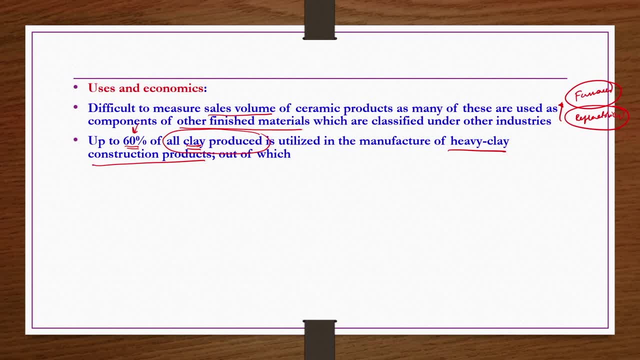 clay that is used for a heavy clay construction products, you know out of which: building brick, sewer pipe and then drain tiles account for 38 percent. 19 percent account for Portland. cement light weight aggregates account for 10 percent right. 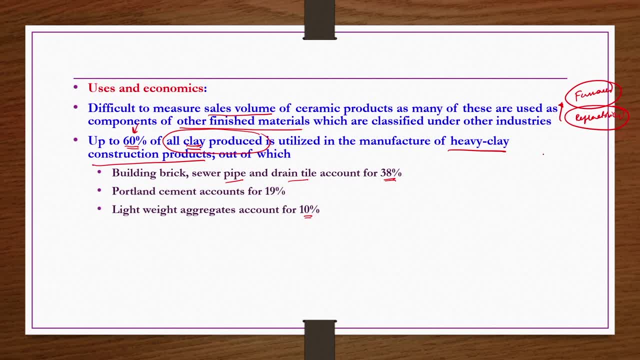 And more examples, under these cases, of products of ceramic industries. or you know, ingredients of ceramic industries are used in some other industry or, like you know, they include paper and pulp industry, cement industry, glass industry, Right, You know so many things associated with the ceramic industries. they are also associated. 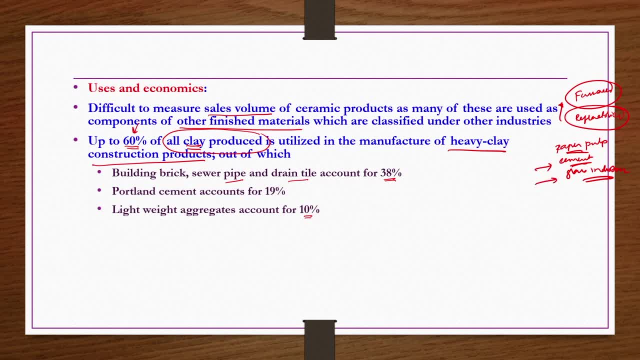 with the cement and glass industry And the same you can realize as we progress ahead into the course of ceramic industries. Refractories also use large quantities of clays. clays are also used as fillers in many products such as paper, rubber, plastics, paints and fertilizers. some clays are also 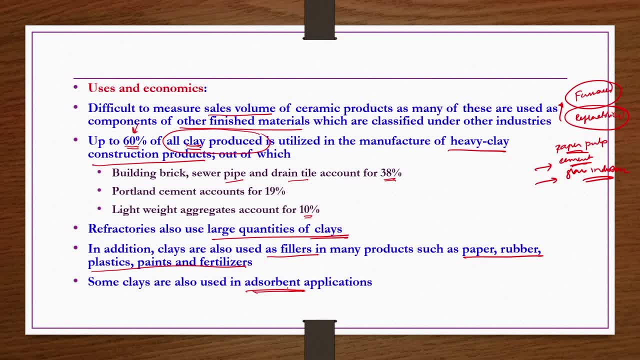 used in adsorption, Adsorbent applications like silica, etc. they are also used as adsorbent, and then silica is one of the important component of a ceramic industry. Other applications include drilling mud, floor and wall tiles, pelletizing, iron ore pottery. 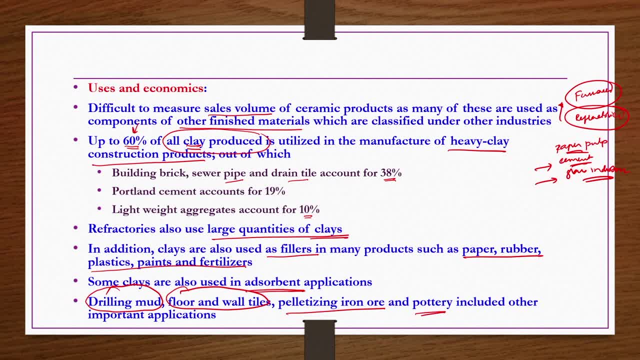 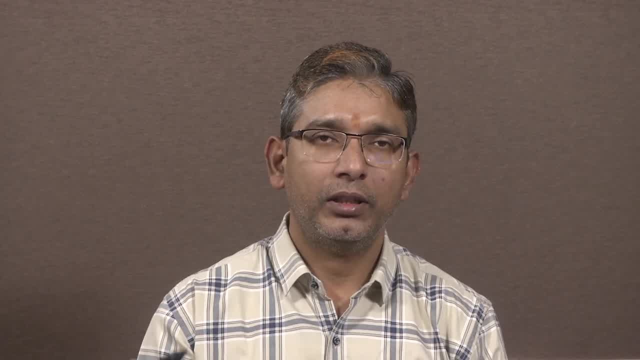 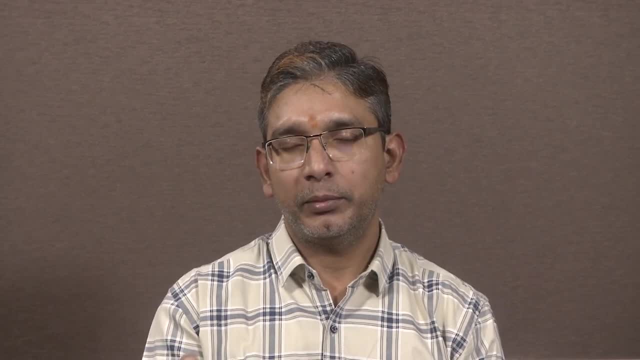 etc. all they may be included in the uses and applications of ceramic industries. Now we have seen a few basics of ceramic industries, and then what are the different types of characteristics that you expect from a given ceramic product? and then what are the different types of ceramic? 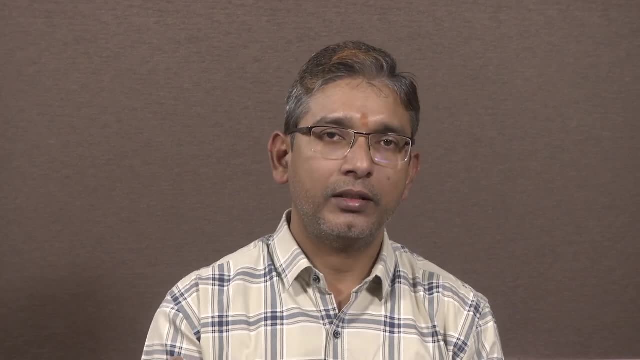 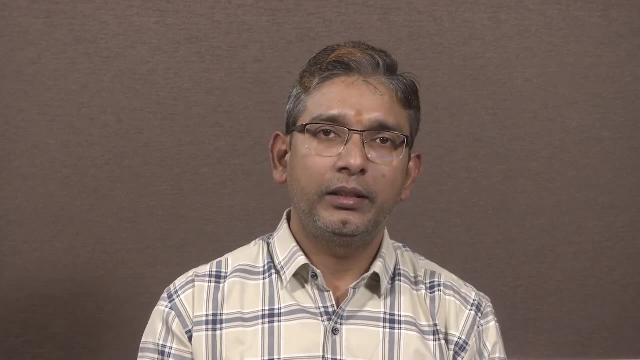 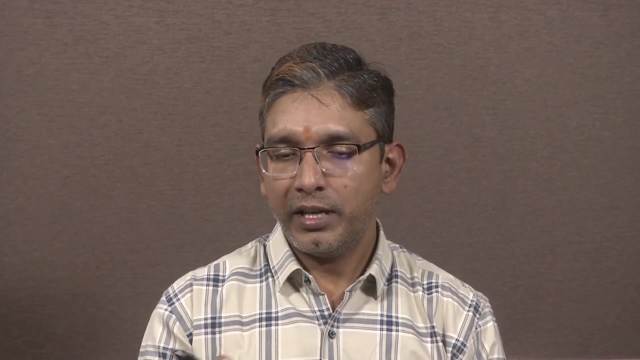 products are possible etc. applications, uses etc. those things we have seen. Now we see basic raw materials of the ceramic industry. This particular lecture is targeted primarily on basic raw materials and then basic ceramic chemistry. So first part of the lecture we are going to start now, that is on basic raw material. 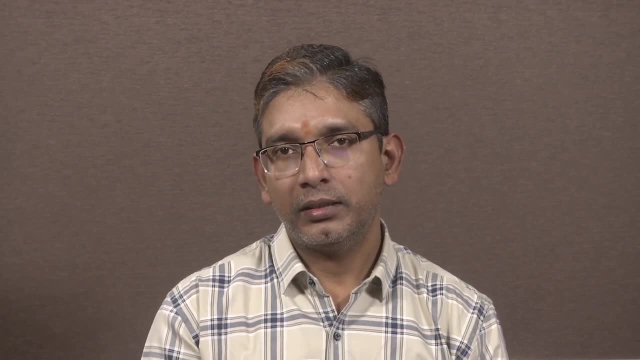 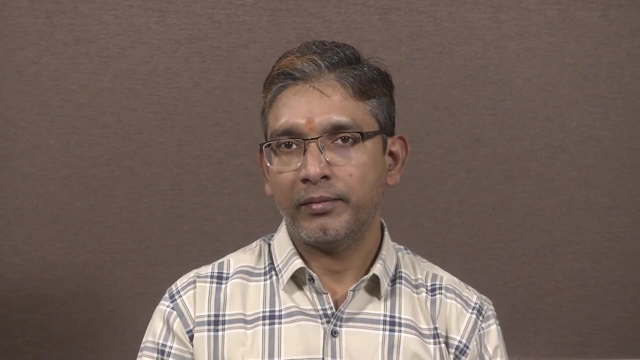 Why are we discussing so much about the raw materials? Because that we are going to realize, in almost all ceramic products, clay is one of the important raw material. Then, along with that one, there are other raw materials, like you know, sand, feldspar. 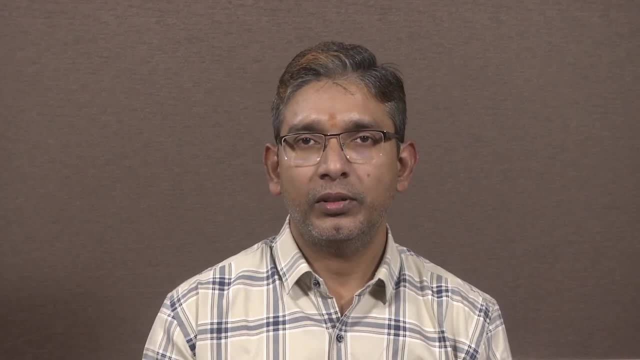 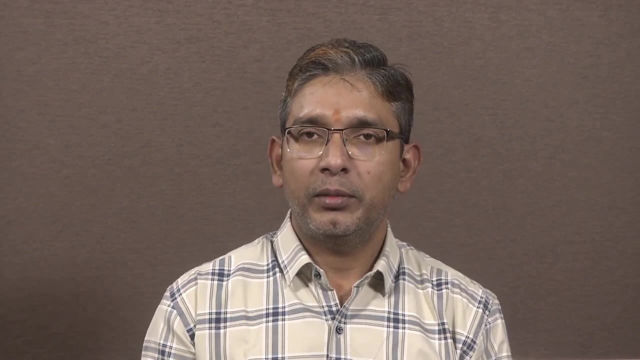 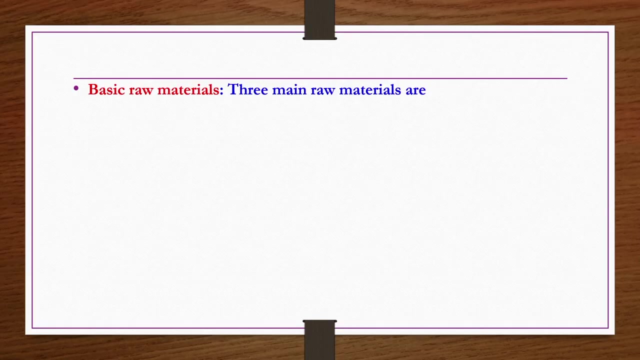 etc. are there. That is the reason it is very much essential to understand or learn a few basics about such raw materials as well. rather simply mentioning these are the raw materials utilized for production of several ceramic products. It is important to understand their basic chemistry. 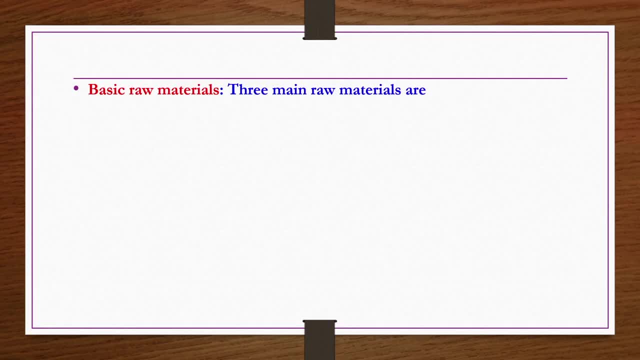 So basic raw materials of ceramic industry. three main raw materials are very common in any of the ceramic product that you take. So one of them is clay. another one is the feldspar. third one is the sand. Primary source of feldspar mineral is igneous rocks. 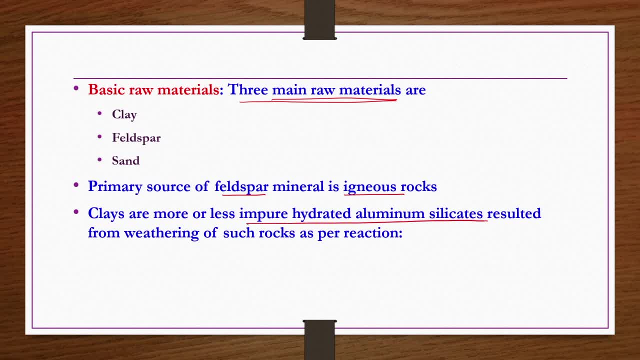 Clays are more or less impure. hydrated aluminum silicates resulted from withering of such rocks, as per the reaction given below. That is, if you take potash, feldspar, actually feldspar- different types of feldspars are there. 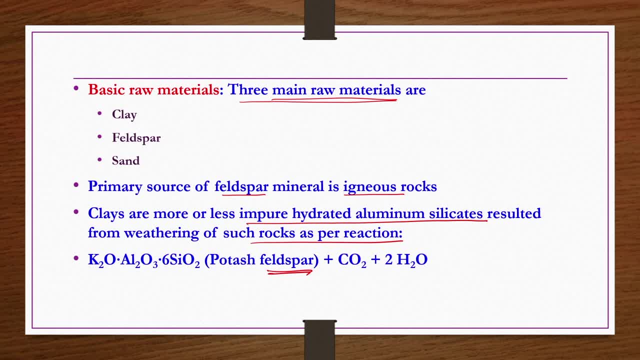 Potash feldspar, and then soda feldspar, lime feldspar, etc. that based on the feldspar. you know Al2O3, SiO2 are common, and then third one, whatever is there. based on that one, the name is given. 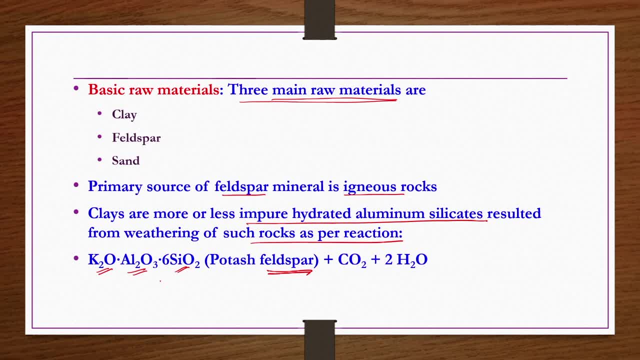 Now here, K2O is there, so that is the reason this feldspar is having the name of potash feldspar. It reacts with carbon dioxide and water at high temperatures. Then you get a clay mineral. one of the clay mineral is kaolinite, which is having the formula. 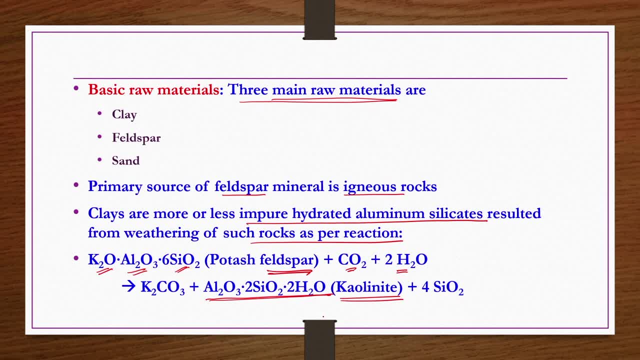 Al2O3 to SiO2 to H2O. This is one of the raw material from, or one of, the clay mineral that is required for almost all ceramic products production. So when this reaction takes place, along with the potassium carbonate and then silica, you 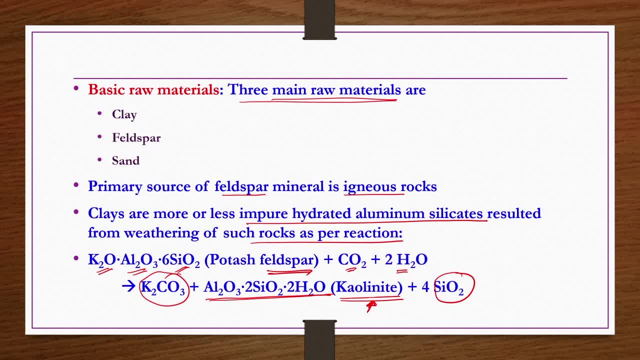 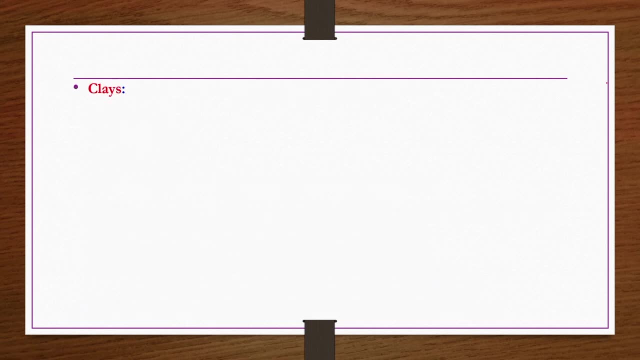 get a clay mineral. So this is the reaction: The clay mineral, kaolinite, which is very essential for most of the ceramic products manufacturing. So now what we do? we discuss individually about each of them. Now we talk about clays. Clays are primarily having several types of minerals. 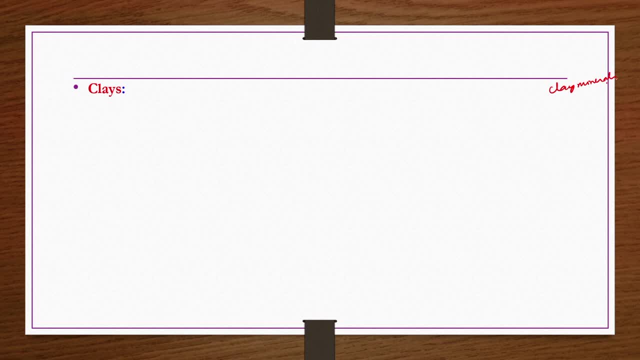 They are also known as the clay minerals. These minerals include several types of inorganic oxides, Primarily inorganic oxides, But the clay mineral oxides should be there. Some of them may be important for a given application of ceramic industry. 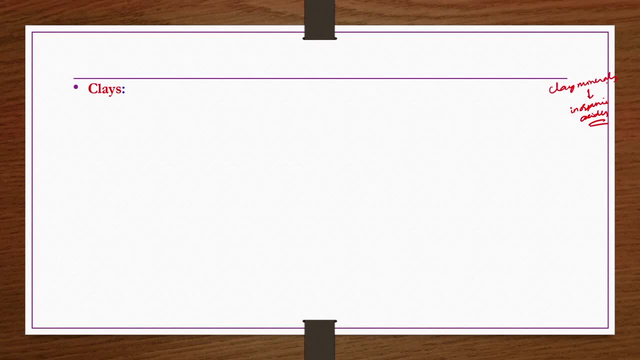 Some of them are important for the given application of glass industry. Some of them are may be important for the given application of cement industry. like that are there. So what we have to do, We have to do a kind of a clay upgrading so that to get the required minerals, which are 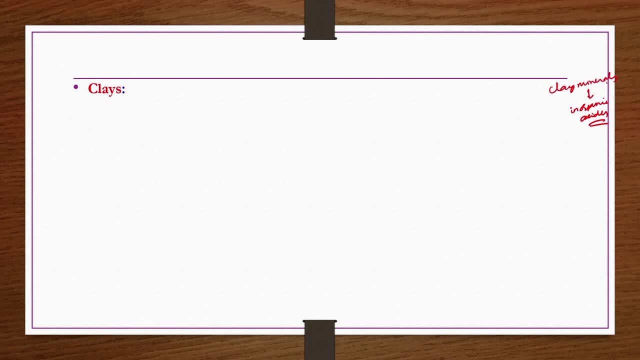 essential from the ceramic products making point of view. Okay, So number of mineral species are available which are known as clay minerals. These mainly contain mixtures of kaolinite, which is having formula Al2O3, 2SiO2, 2H2O. 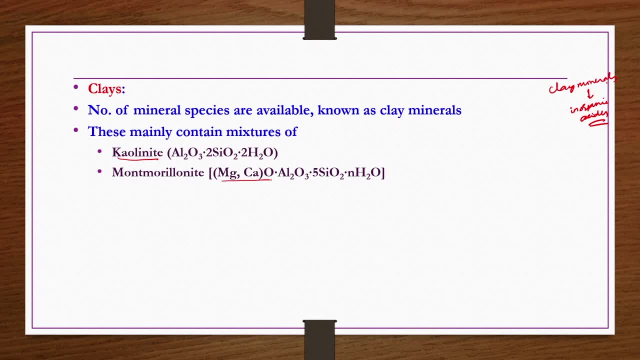 Then montmorillonite, which is nothing but MgO, Al2O3- 5SiO2 NH2O, or CaO- Al2O3- 5SiO2 NH2O. Then third one is illite, which contains variable amounts of K2O, MgO, Al2O3, SiO2 H2O. 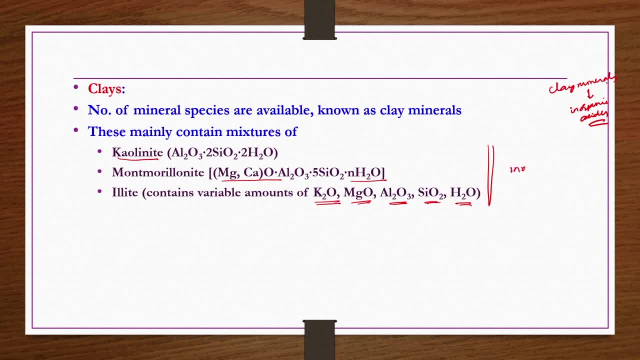 Now you see, all of them are inorganic oxides, except this H2O component, because H2O is coming, because these are hydrated. So you see primarily inorganic oxides only. So clays primarily consisting of inorganic oxides, so out of which this kaolinite is. 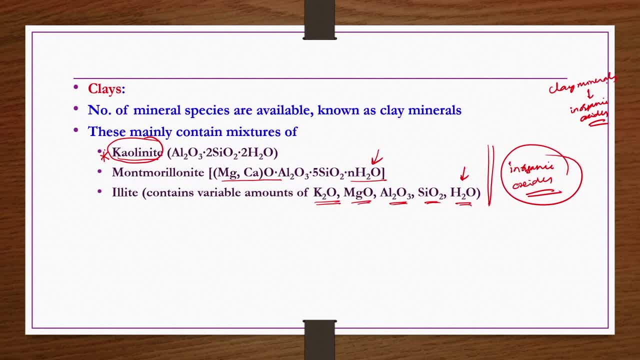 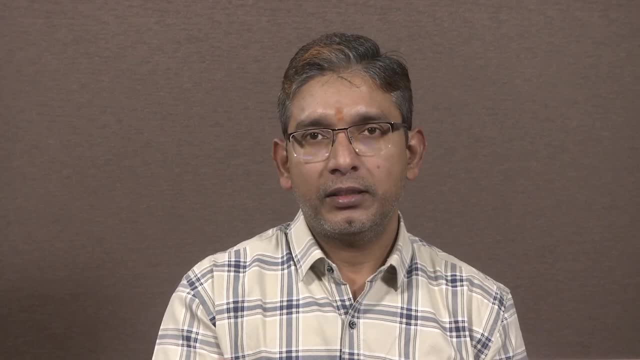 used To larger extent to produce different types of inorganic, different types of ceramic products. From ceramic industry viewpoint, clays are plastic and moldable. you know they should be moldable. Actually, these clays, etc, feldspar, etc. and then sand etc. you take together and 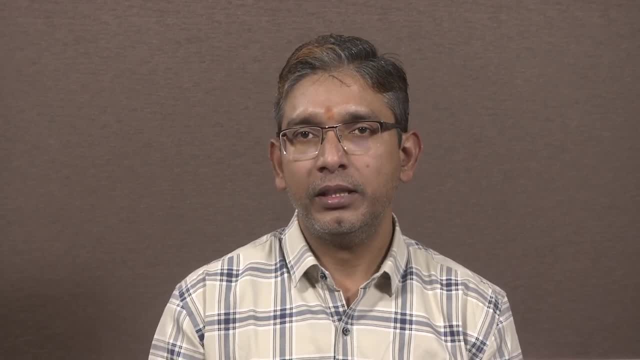 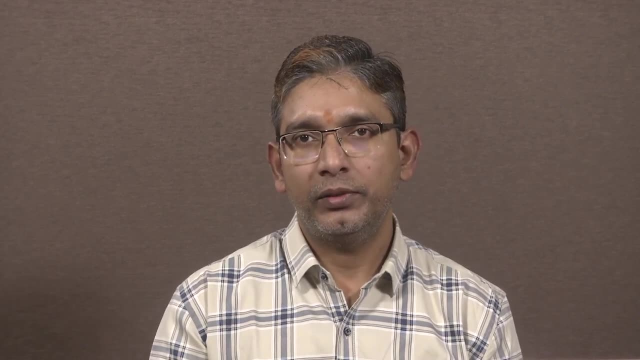 then you heat it to the higher temperature. so certain reactions taking place, right? So those things we are going to see anyway. So when such reactions takes place, you get a, you know, liquefied sample, It should be in a moldable conditions, right? 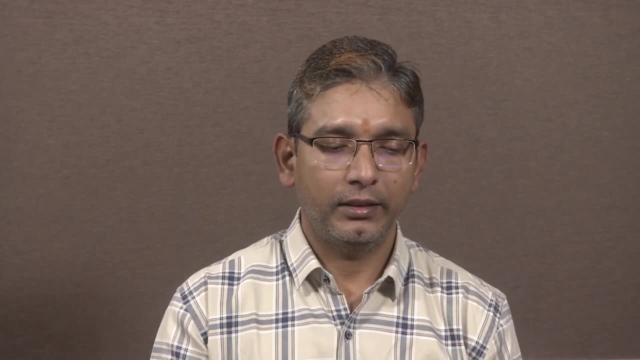 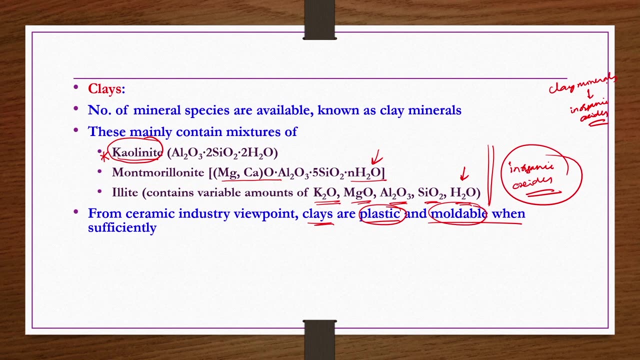 So that you know you can make a required product shape, and then you know design etc. So clays should be plastic and they should be moldable. when sufficiently high temperature is supplied to those clays, Then only it is a good one for production of certain kind of ceramic products okay. 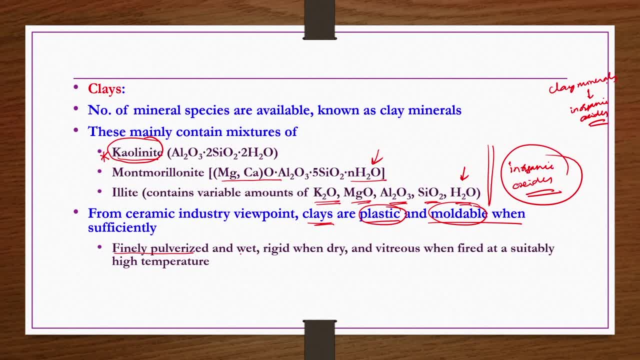 So these clays should be finely pulverized and then wet. They should be wettable, right, Because without, if they are not wettable, it is going to be very difficult to make a product of required shape, right. And then when they dry, they should be rigid. and then when you fire them at high temperature, 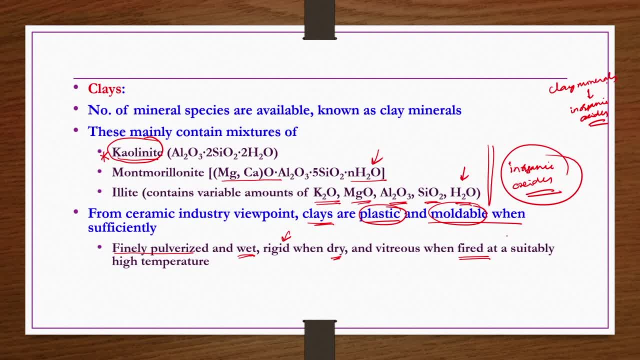 or calcine them at high temperature like 1200, 1400 degree centigrade. they should be wettrious, okay. So from the ceramic industry viewpoint, clay should be plastic and moldable when sufficiently finely pulverized and wet. 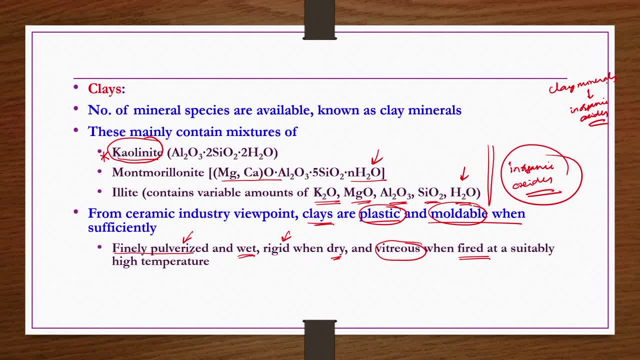 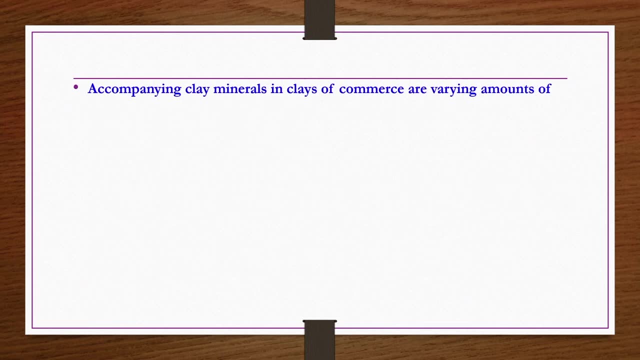 Rigid when dry and wettable, Serious when fired at a suitably high temperature. Most importantly, manufacturing process depend upon these properties of clays. So all these properties we are going to discuss from the product point of view. So now, what are these? clay minerals in general include? 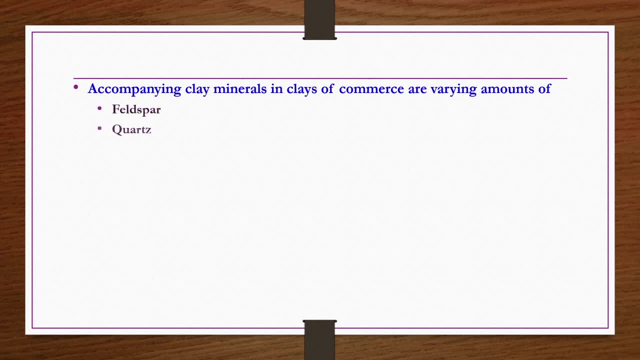 They include varying amounts of feldspar, quartz and then other impurities such as iron oxides. okay, So obviously when you have impurities you know They should be removed. They may not be impurities for other industry, like metallurgical industry or something like. 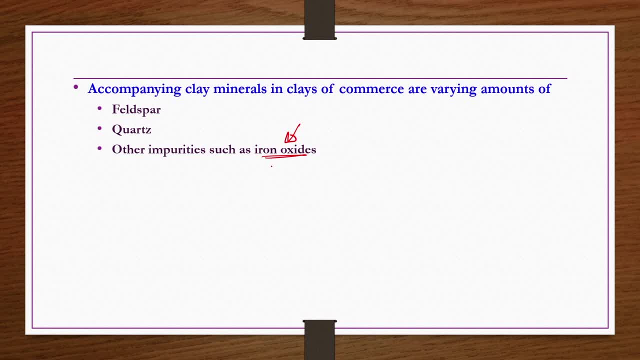 that, But they are impurities. as far as you know, we are concerned about the ceramic industries. So now, from the ceramic industries point of view, such impurities should be removed. Other kind of impurities may include, like mica etc. They should be removed. 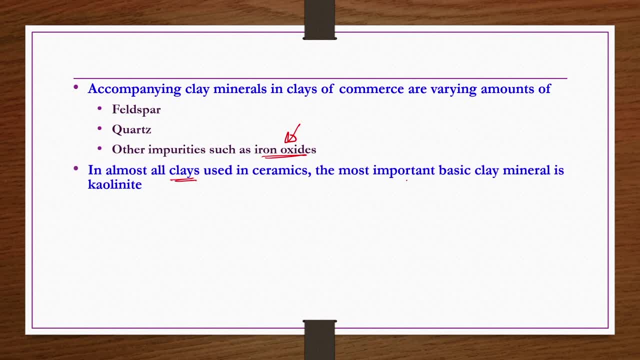 In almost all clays used in ceramics. the most important basic clay mineral is kaolinite. This is very much essential, okay, Okay. However, very high plasticity is desired. bentonite clays based on montmorillonite are used to. 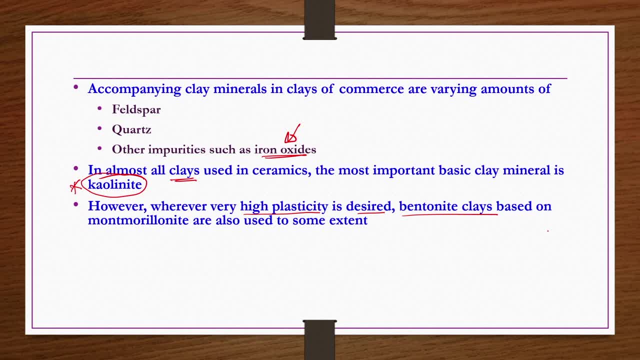 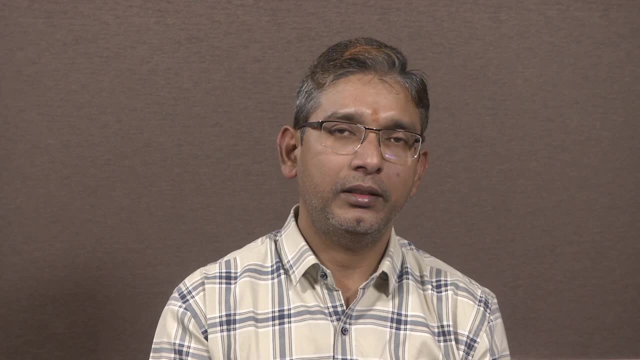 some extent. What do you mean by actually high plasticity and then high workability or moldability? When you apply high temperature to the raw materials mixture they become liquid kind of products and then they should have proper flowability etc. So then we can say that the material is having, you know, workable kind of conditions. okay, 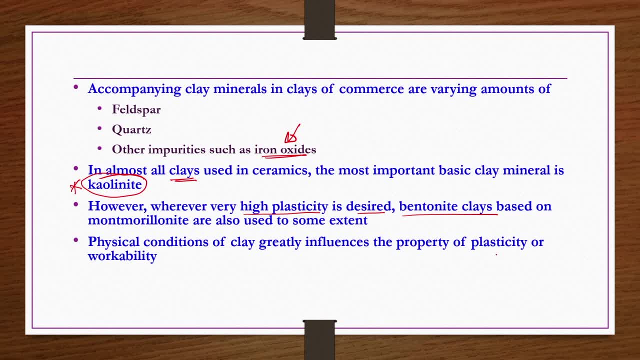 Physical conditions. Physical conditions of clay greatly influence the property of plasticity or workability, definitely. And then the influence varies among different types of clays, One clays to other clays. whatever the influence of this clays is there. so that is going to. 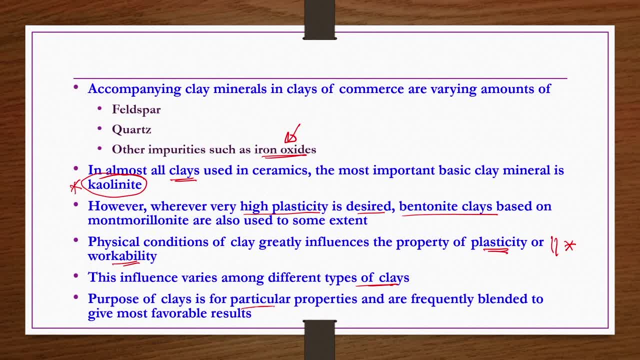 be changing. Purpose of clays is for particular properties and are frequently blended to give most favorable results. Different clays are used. actually, Though we are calling like, kaolinite is used. Okay, It is one of the mostly used clay in ceramic industry, but other types of clays are also. 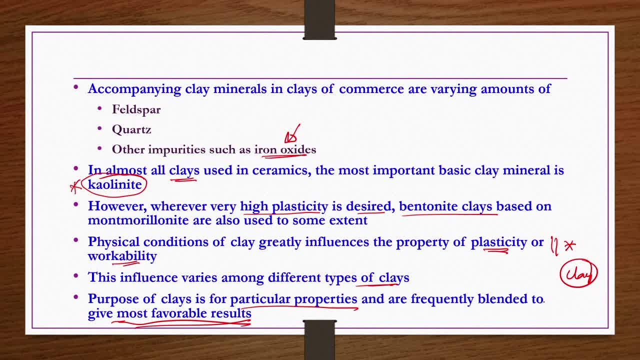 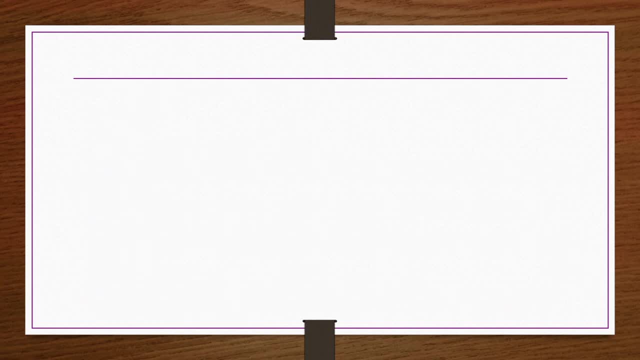 there right, So they are also used. You know each one is having certain kind of- you know- applications, certain kind of characteristics. But it has been found that when you mix them frequently, you know blend them, so then you get most favorable results from the product point of view. 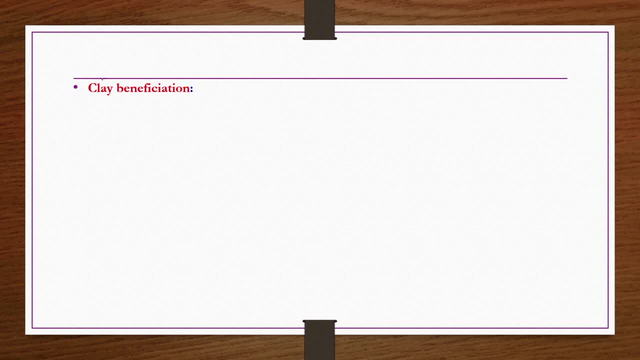 So, as we have already seen the clays that we are having, You know It is having impurities, Impurities like sand, mica, iron oxide, etc. So they have to be removed. Removal of these impurities from the clay is known as clay beneficiation. 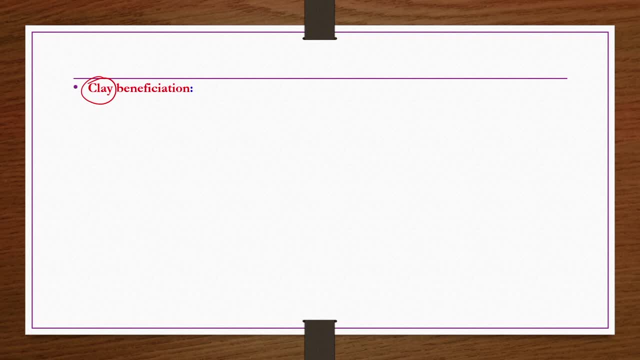 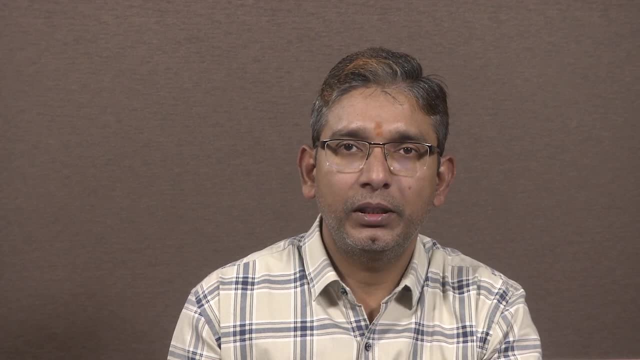 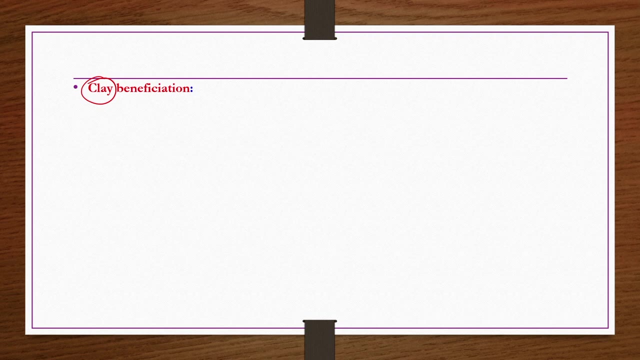 We are not calling clay purification, because clay is not one single component that we are purifying. It is a combination of different components, right So. but, however, from this mixture of different components we are removing some of the impurities. They are impurities from the ceramic industry point of view only. otherwise, those impurities, 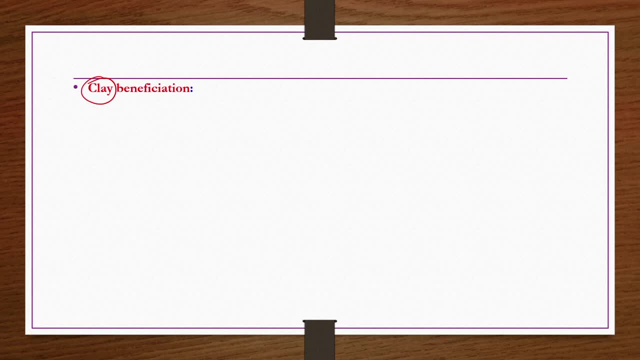 after removal they can also be used in some other applications. Let us say iron oxide: if you are producing in a good quantity, so you can use it in metallurgical industry. Let us say mica impurity: you are separating in a large quantity, so that should be sent. 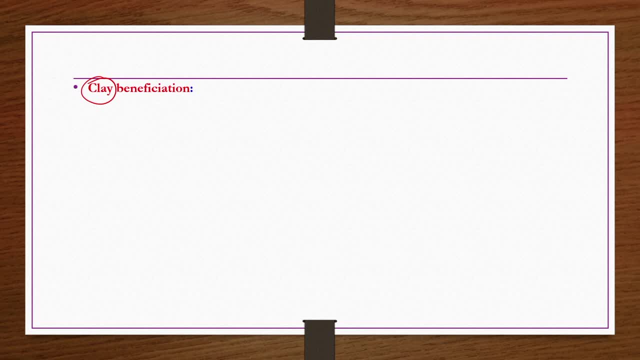 to the mica plant for a proper utilization point of view They are impurities. from the ceramic industry point of view only, Clays differ very much in their physical properties and impurities present in clays. thus often it is necessary to do upgrading of clays, upgrading in the sense removing unnecessary 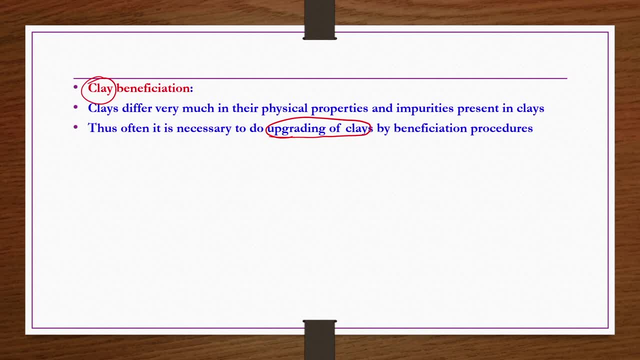 or undesired components from the clays. So this upgrading is done by beneficiation process, which is primarily includes unit operations. only Whenever we have beneficiation, etc. you can clearly understand that there is a need for there is a float, rotation is possible. there is a size separation is possible, thickening, 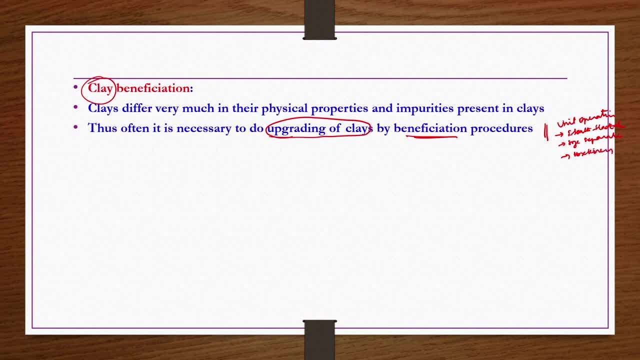 is possible. So all of these things are unit operations only. So what you understand? not only this: clay beneficiation, upcoming sections of production of different types of clay products. you see, primarily unit operations are only involved. okay, Only sand and mica are removed from clay by their beneficiation. china clay beneficiation. 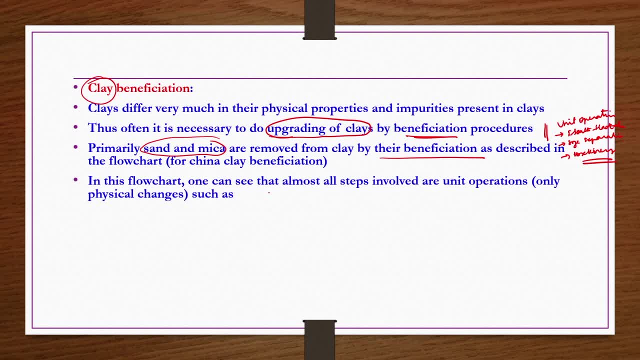 flow chart we are going to discuss in the next slide. anyway. Here one can see that almost all steps involved in the china clay beneficiation are unit operations only. There are no chemical reactions, There are only physical changes. are there, okay? Physical changes? size separation is one thing that you can definitely expect in separations. 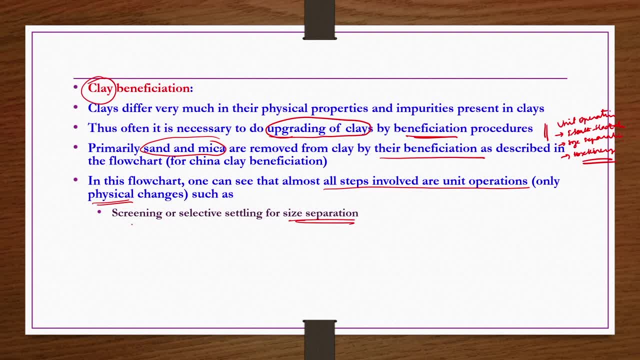 or you know, beneficiation of ore etc. And that is done by the screening or selective settling for the size separation, and then filtration would be there to filter out the unnecessary things. okay, Then after filtration, you definitely need to dry the material before processing to the 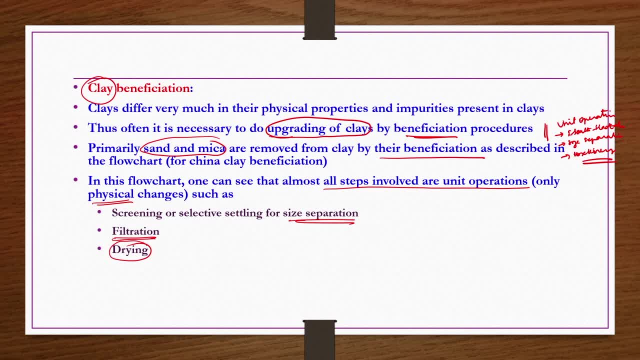 next level, okay, And there may be other kind of unit operations, like you know, thickener, etc. hydrostatic separators or magnetic separators, etc. those things may also be possible. So we have listed only a few. In this process, colloidal properties are controlled by appropriate additives, such as sodium silicate. 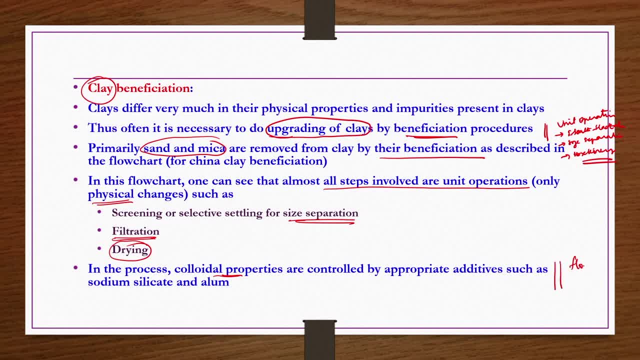 and alum. You need to have a flocculating agents etc. you need to have a deflocculating agents, etc. in the process. So they are required to maintain the colloidal properties. okay, So those things we are going to see. 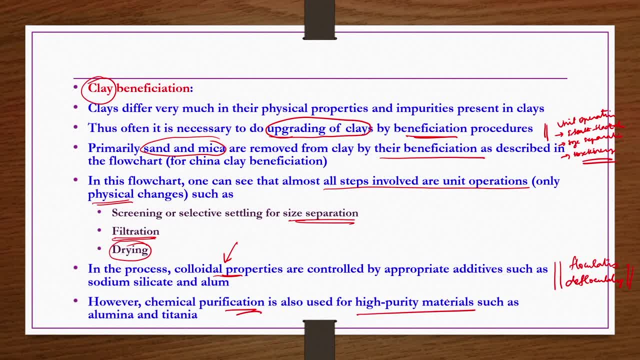 However, chemical purification is also used for high purity materials such as, like you need to produce pure alumina or pure silicon, Then you can go for a chemical purification. okay, But majorly- most of the clay products you know, you do not need to go for a chemical. 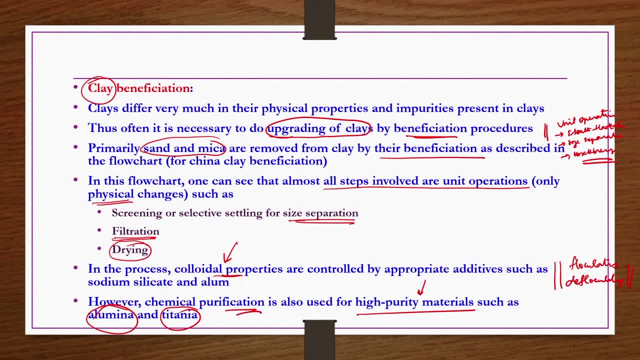 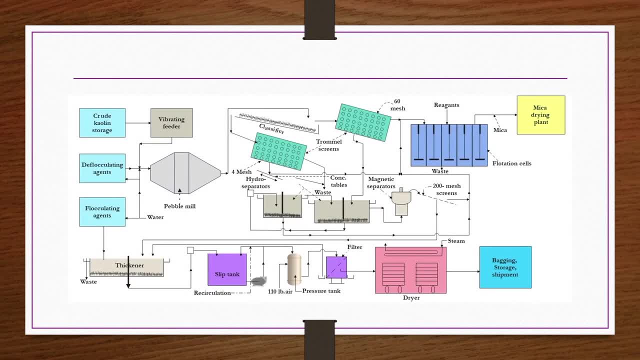 purification of clays. You can go for a clay beneficiation which is done by several physical steps or unit operation steps. Now, here we see, the flowchart for the china clay beneficiation. Okay, So this is the flowchart. Okay, Here what we have. we have a pebble mill, right? 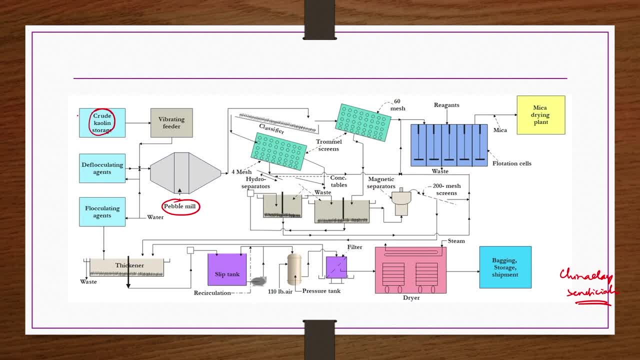 To this one. we are feeding crude kaolin from the crude kaolin storage through a vibrating feeder. Why vibrating feeder? Because these may be having of different sizes right, And then may not able to pass easily through the columns or, you know, pipes etc. so then 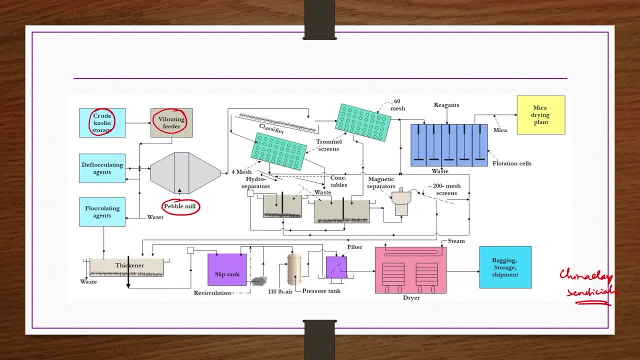 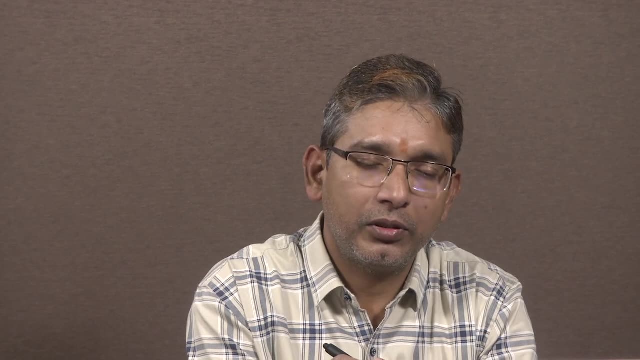 a vibrator is provided, Provided to the feeder, so that you know, vibration will enhance the movement of this particulate matter. Usually, particulate matter does not flow down easily, even if it is by the gravity or by pressure or whatever. So you know, storage and transport of solids is very difficult task. 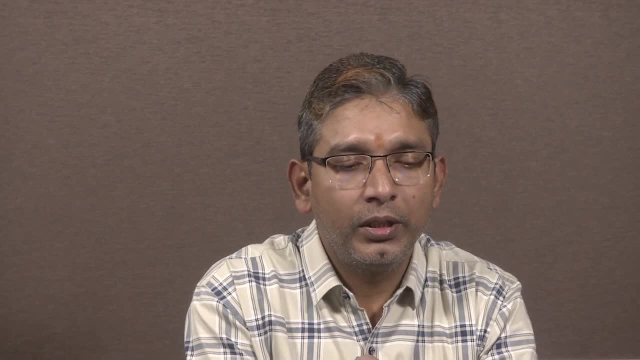 So for that reason, you know, vibrating feeders are often used to transport the solid materials. So this crude kaolin is fed to the pebble mill through a vibrating feeder. So this crude kaolin is fed to the pebble mill through a vibrating feeder. 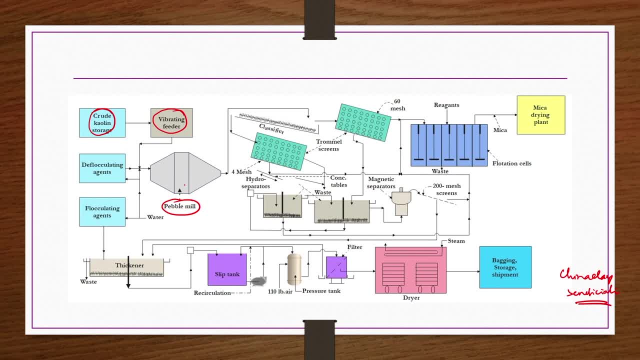 So this crude kaolin is fed to the pebble mill through a vibrating feeder. Okay, To this one you are also giving deflocculating agents, because these crude kaolin storage whatever is there from that, the material that you take that may be wet or bit damp. 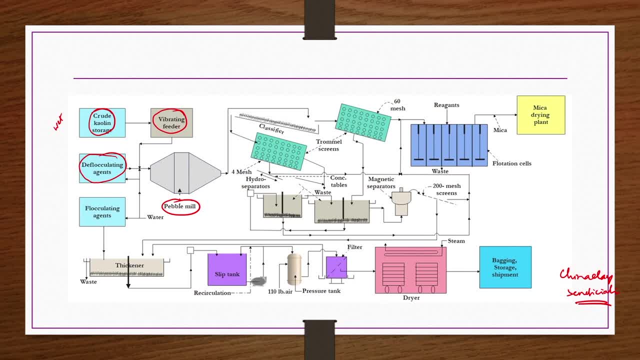 If it is wet or damp, so it may not flow through easily. So for that reason also you need to have a vibrating feeder. If it is wet or damp, then what happens, you know, when the material is taken to the pebble mill. 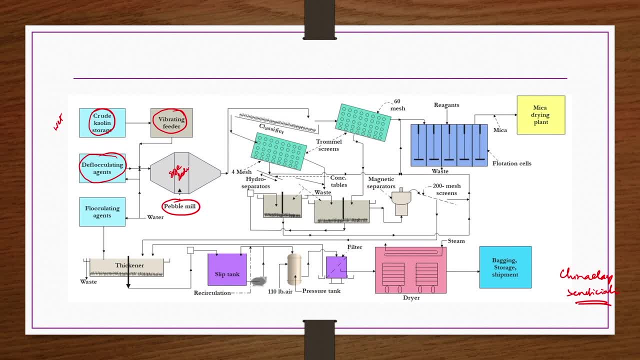 If it is wet, size reduction is taking place. That will also not be efficient if the material is wet, because if it is wet you know they may form lumps kind of thing. So when it is forming lumps, or rather size reduction taking place, breaking of lumps. 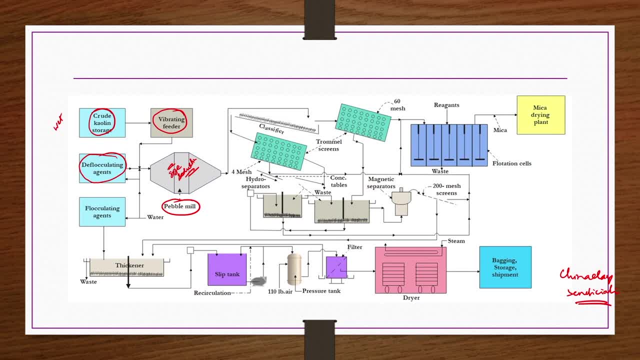 will only be taking place, or most of the energy utilized for the size reduction would be utilized for the lumps breaking, which is not at all required. So for that reason, there are some deflocculating agents. are, you know, provided. So these deflocculating agents are provided. 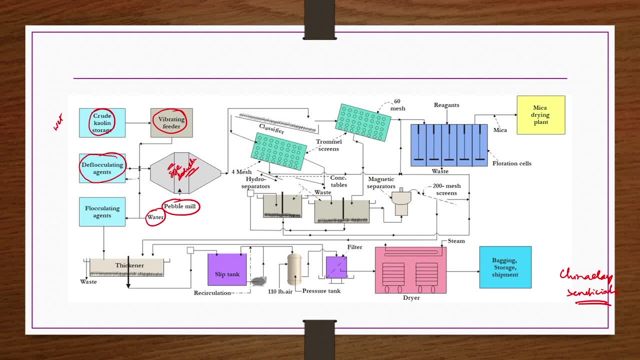 Okay, So this pebble mill is nothing but a cylindrical container which will be rotating, and then rotational speed should be such a way that it should not be more than the critical speed. Critical speed is the one, you know, at which the centrifugal forces are balanced by the 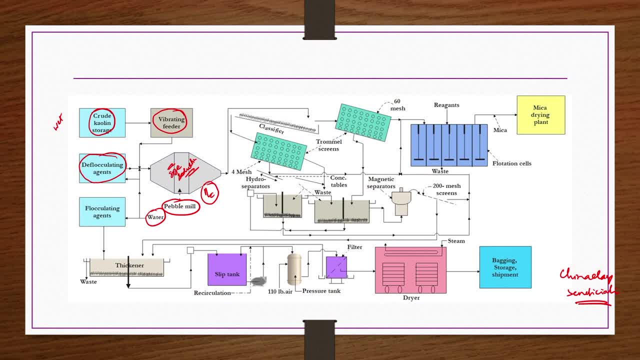 gravity force. So your rotational speed has to be less than the speed at which centrifugal force is balanced. So the centrifugal force is balanced by the gravity force acting on the material that has been fed to this rotating drum. right, This pebble mill is nothing but rotating drum, where you can visualize as a rotating drum. 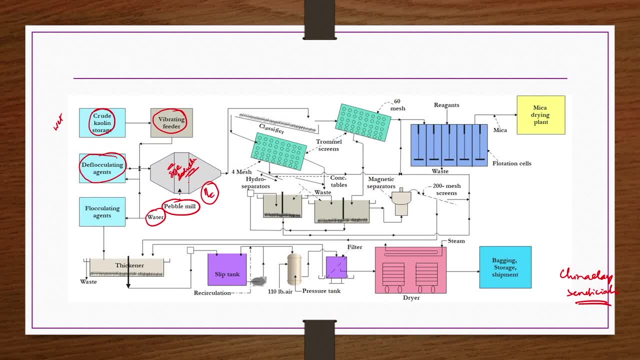 To this drum. you have taken pebble. If it is a ball mill, you will be taking a balls, steel balls or, you know, wooden balls, etc. If it is a rod mill, so then you may be having metallic rods or wooden rods, etc may be there. 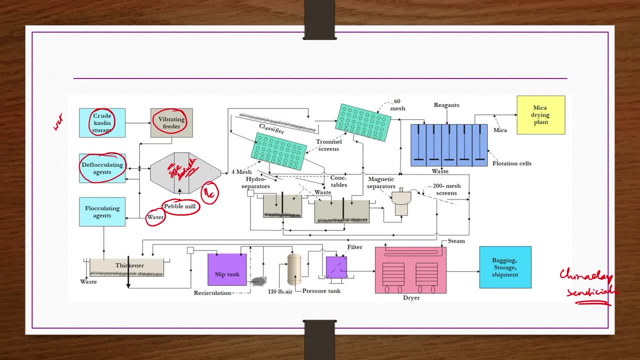 as a kind of, you know, grinding medium. Now, here it is a pebble mill, So then pebbles of different sizes, So pebbles of different sizes, of different nature, would be taken into the material as a grinding medium To this one. when the material, whatever the kavelin, is there, that comes in right. 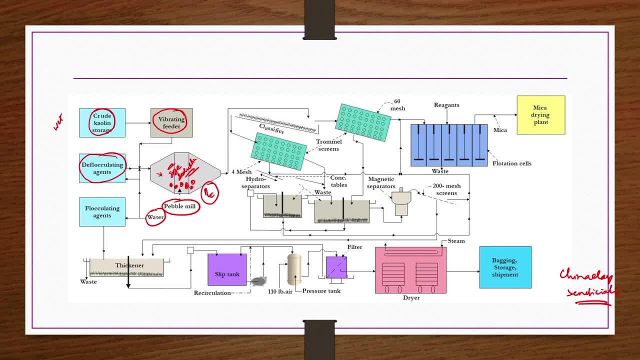 So, and then when it rotates, moment the rotation takes place, the material- whichever was there at the bottom that will be- gradually moves up, and then, moment it reaches the top location, the material will fall down. Now the material is the combination of the feed material plus these pebbles. 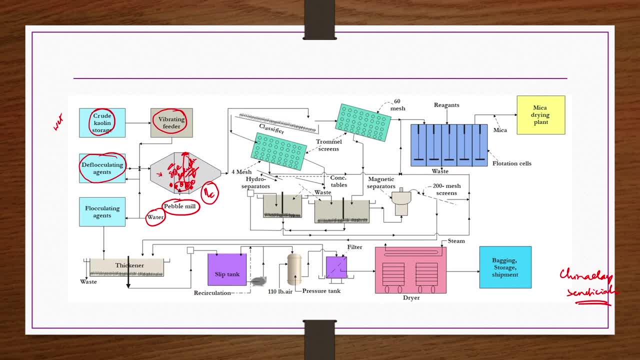 So when they fall down, so a kind of impaction takes place, and then some grinding takes place and then material size reduction takes place, right? So size reduced material will then be passed through different steps of a unit operations like a classification, hydro separation and then concentration tables and magnetic separators. 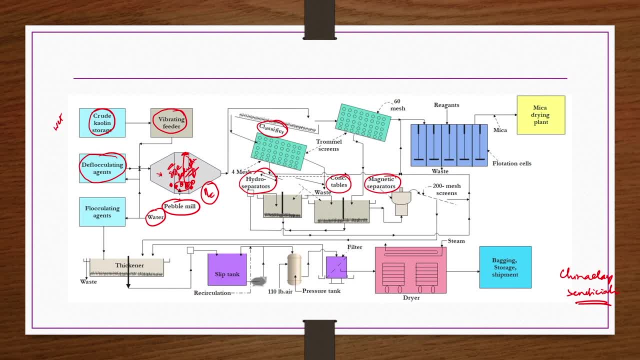 etc. as per the requirement right. So the magnetic separators are usually to catch the materials which are having magnetic properties. When this size reduced material comes and interact with this magnetic separators in the materials, if any material which is having magnetic properties, they will be captured. 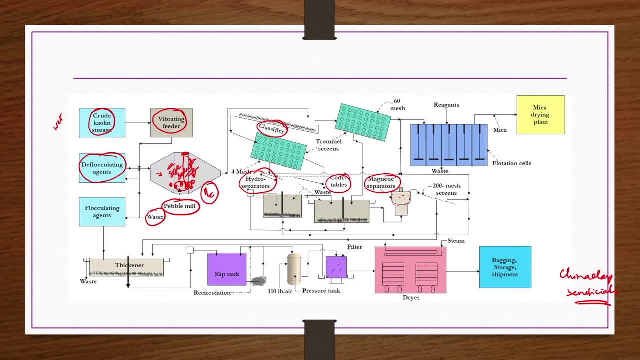 here and then remaining material will be sent forward, right? So here you know, mesh sizes or different mesh sizes are there as per the requirement. you know this size separation is taken place If you required 60 mesh size, so accordingly, the process would be taken place. 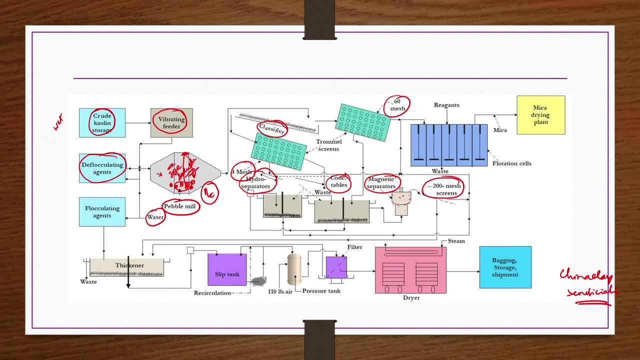 If you need 200 mesh size materials, then accordingly, the steps would be taken. Okay, So these are the steps which should be considered. What do you mean by mesh size? I already explained. Let us say, within a sieve. if you have a sieve like this, 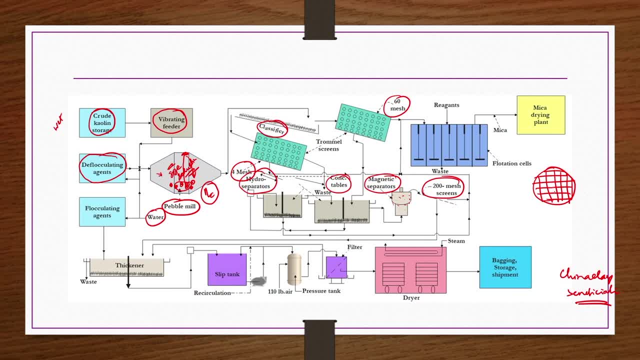 So, within this screen or mesh, you take a one linear inch, one linear inch distance, and then, within that linear inch distance, let us say this is one linear inch distance, Within this one, if you have only four openings: 1,, 2,, 3,, 4,, 5,, 6,, 7,, 8,, 9,, 10,, 11,, 12,, 13,, 14,- 15,, 16,, 17,, 18,, 19,, 20,, 21,, 22,, 23,, 23,, 24,, 24,, 25,, 26,, 27,, 28,, 29,, 30,, 31,, 31,, 32,, 31,, 32,, 33,. 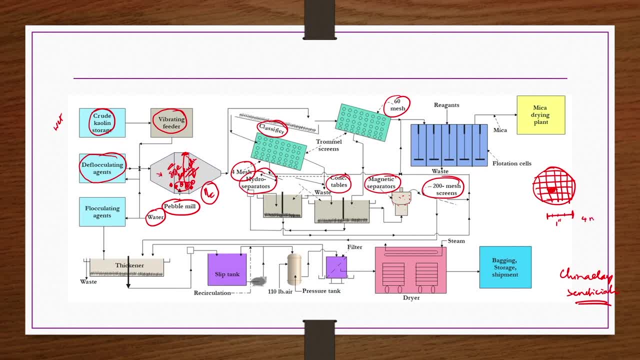 34.. So this is one, 2,, 3,, 4.. So then this is called 4 mesh. So what you see, if the mesh number is smaller, the opening would be bigger. Let us say, if you have a same one linear inch distance here from the screen you have taken. 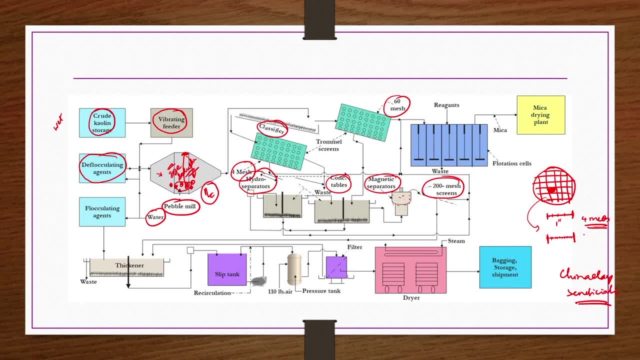 let us say, if you have 60 openings here like this, then this mesh is known as 60 mesh And then obviously the openings would be smaller than the 4 mesh. So 200 mesh- even smaller- would be there, Like you know. 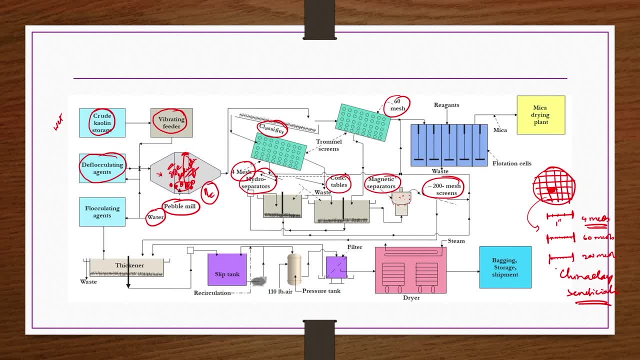 Okay, few micron size opening would be there. okay, So that is what the mesh anyway. So now, after passing these materials, whatever the material that is coming over from the 60 mesh, that is taken to a flotation cell to which reagents or flotation or froth forming. 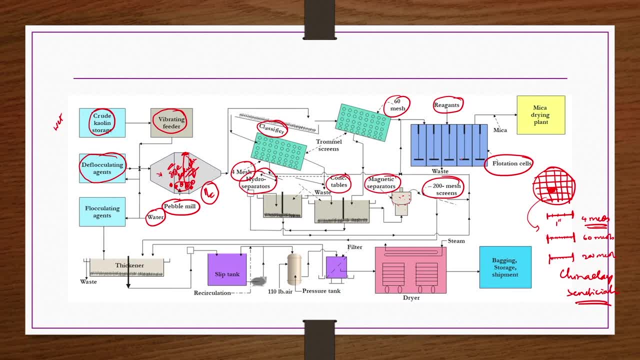 reagents are supplied and then mechanical agitation is also done so that, you know, froth formation takes place and bubbles forms, Bubbles forms and the froth of bubbles, you know, raise to the top of the flotation cell, right So when they raise here. so, whatever the material, 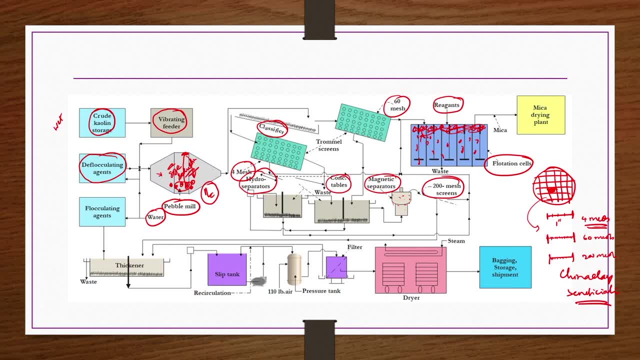 having the lower density, that material will be stick to these bubbles and then they will be floating. So in this case, mica is the one which is having lower density, So that will be attached to the bubbles and then they will be floating on the top. So then they 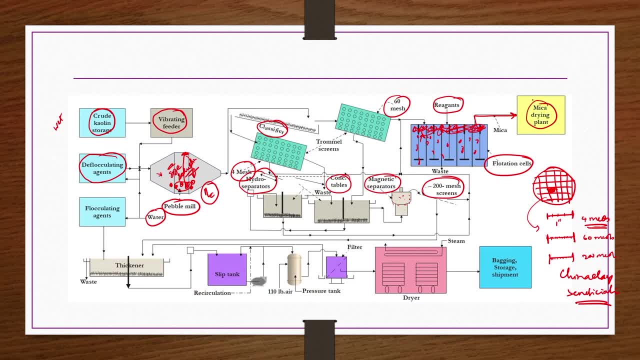 will be separated out and taken to the mica drying plant, Whereas the material which is passed through 200 mesh, which is primarily having the desired clay minerals, you know they will be taken to a thickener here. Here in the thickener are nothing. but you know settling. you know settling by the gravity. So if it is settling, 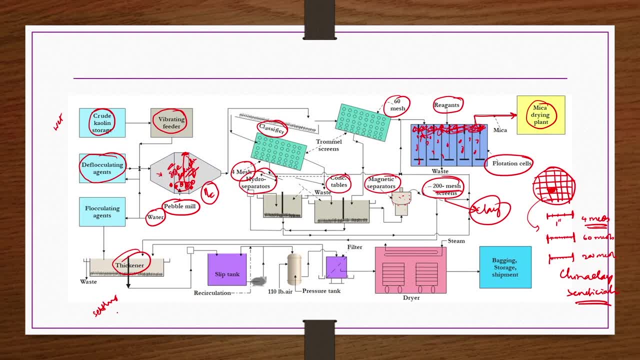 by the gravity. so then gravity thickener. If it is settling by the centrifugal force, then it is known as the centrifugal thickener. okay, So here the wave is moving. The wastage material will be floating: from the top that is taken, and then from the bottom. 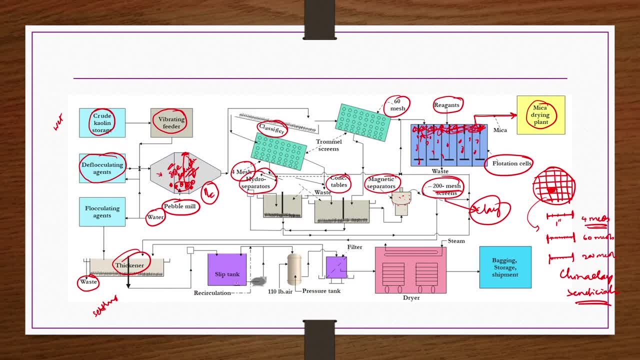 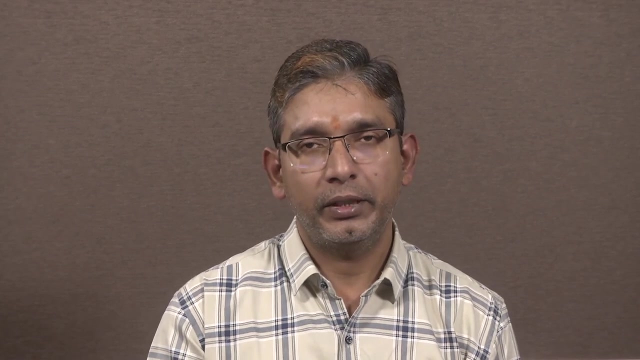 which is the important clay mineral. that will be followed through different sections of pressure filter and then dryer, etc. to get the final clay mineral which has been purified, benefited using physical process, physical changes. There are no chemical reactions at all in this process. okay, That is about the clay beneficiation. 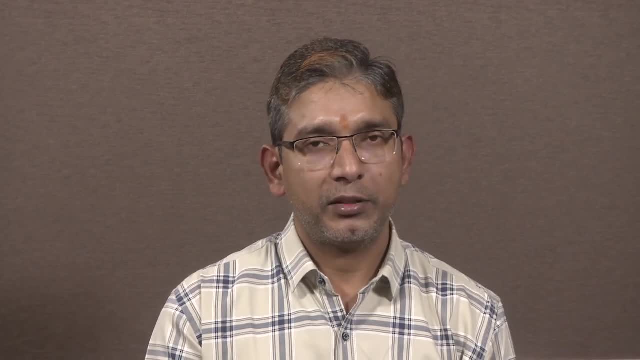 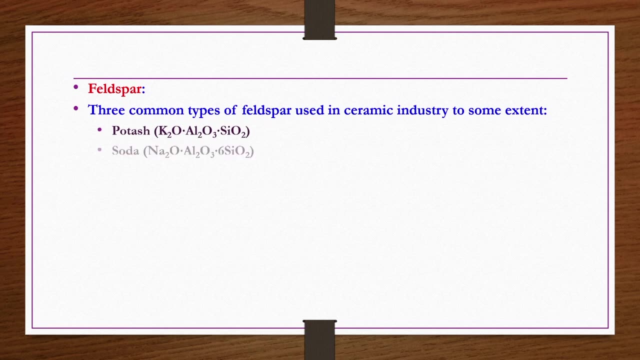 Now we go to the second raw material, that is feldspar. Three common types of feldspar used in ceramic industries. to some extent they are nothing but potash soda. and then lime based feldspar. So potash-based is nothing but K2OAl2O3 because 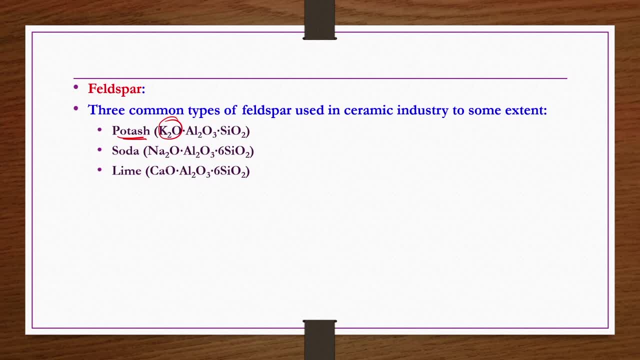 of present, it is known as a potash feldspar, Whereas the soda is having Na2O. that is the reason it is called as soda feldspar, and then the next one is having CaO. that is reason it is known as lime based feldspar. It is primarily good as fluxing constituent. 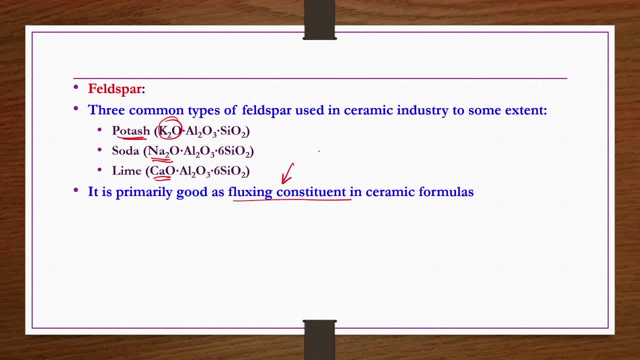 in the ceramic formulas. What do you mean by fluxing? You know they reduce these components, reduce the temperature of reaction or vitrification temperature. You need to do some kind of vitrification Now most of the ceramic products. if you see a kind of glassy, shining kind of appearance. 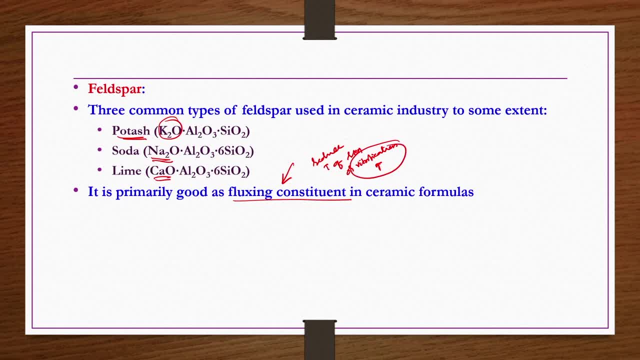 you have. that is because of the vitrification, So that the vitrification is usually can be done at high temperatures for most of the ceramic products. But if you have a good fluxing constituents the temperature would be reduced. That is the reason these components some 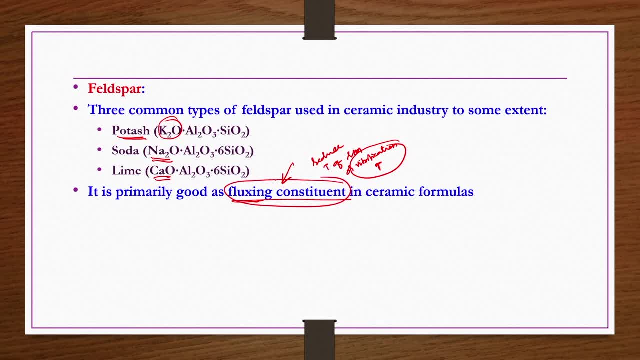 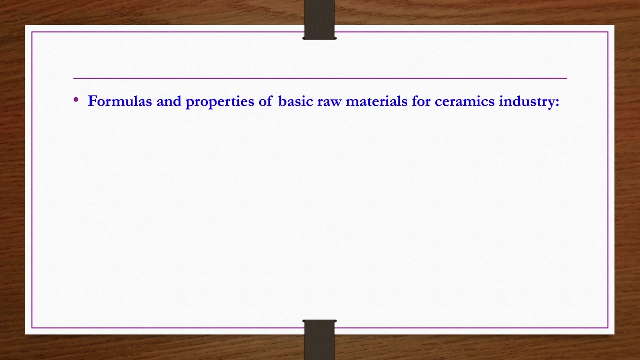 of these components are known as the fluxing constituents in ceramic product formulas. It may present in the clay as mined or may be added as needed. Third important raw material is sand or flint. For light colored products, sand with a low iron content should be used. Now we see formulas and properties of basic raw materials for ceramic industry. 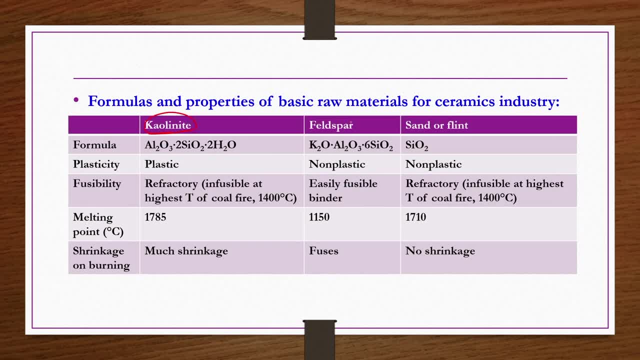 So from the clay minerals we take kaolinite. from the feldspar we take potash, feldspar, and then sand is the other one we are taking. Formula, plasticity, fusibility, melting point and shrinkage and burning are discussed here. 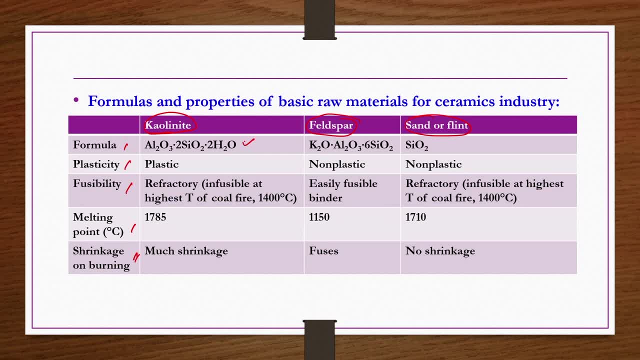 So kaolinite formula. we already know that Al2O3, 2SiO2, 2H2O- It is plastic in nature. So it is a good one, because most of the ceramic materials, or you know, raw materials of the 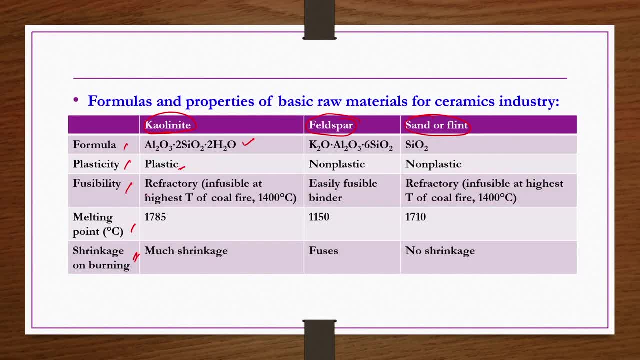 ceramic industry. they should be plastic. And then fusibility. they are of refractory nature because they are not fusible even at the temperature of 1400 degree centigrade. Why they are not fusible even at this temperature? because their melting point is 1785 degree centigrade. So 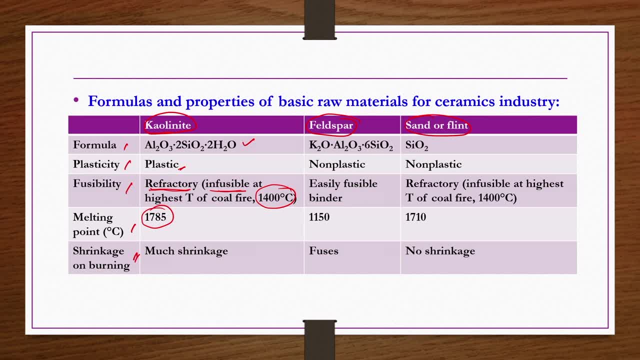 that is the reason. So kaolinite formula: we already know that Al2O3,, 2SiO2, 2H2O It is not a very toxic material Since they will effect the thermal life color. But the understanding of waivers has changed as well. 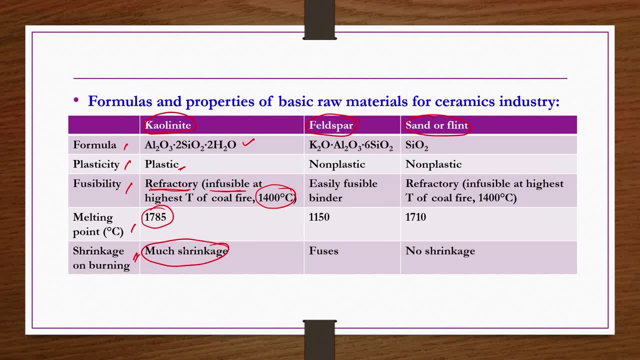 But the problem is that on burning they undergo much shrinkage. You know, thectica is 80 %. if you think that you know melting point is very high, and then it is infeasible even at 1400 degree centigrade. If you think that you take most of the raw, 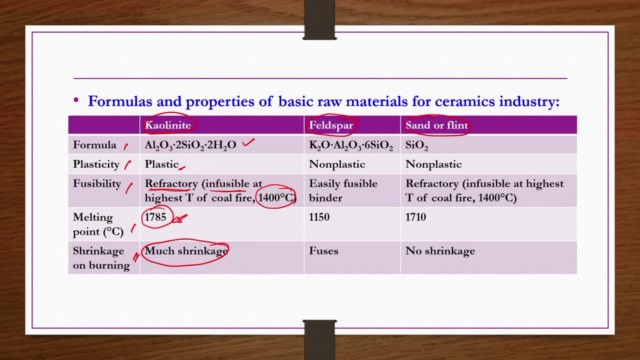 material as kaolinite. Let us say 80% you take kaolinite and remaining 25% feldspar as sand. if you take, You know you may not get a final product. You may have a thermosate противocopium. you takeencarnation by feeding the cofactors with this vessel in blood. If the cofactors are frozen, this will also cause� cust. This is good for covering the 혹시 there, but you just have to take care for discolytic and you will get coacht streptococcus and 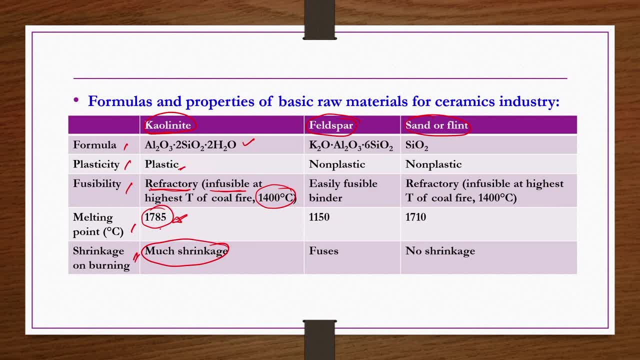 final product. you may have a thermally stable product, but you may not have a proper product, because on heating, you know, kaolinite undergoes a much shrinkage, which is not good. okay. So feldsperr formula is K2O, Al2O3, 6SiO2, it is a non-plastic but it is easily fusible. 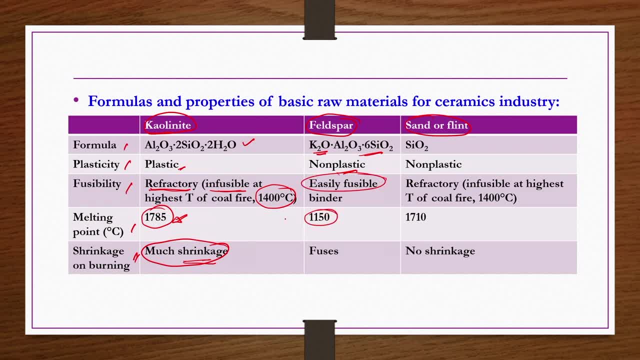 Why it is easily fusible, Because its melting point is 1150 degree centigrade only. right So, but it fuses does not mean that it is not good. when it fuses what it does, it acts as a binder. it acts as a binder and then keep the components tied together themselves, right. 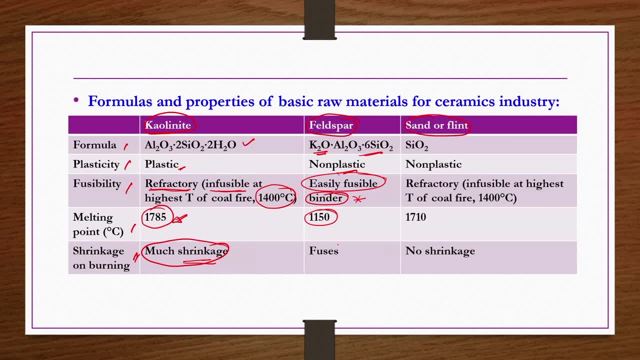 So it is not the fusibility that you have to see, but also other parameters also. you have to see, and then on heating it fuses rather shrinking, okay. Third one is the sand, which is SiO2, it is a non-plastic and it is a refractory, because 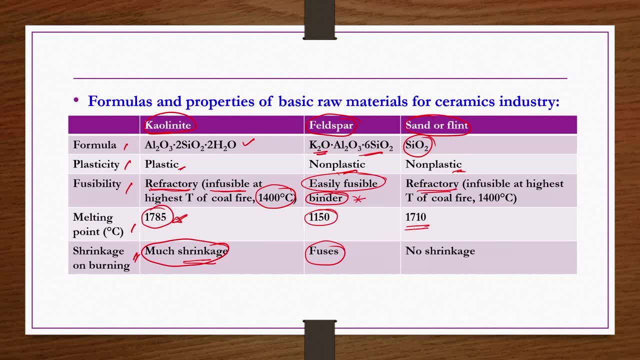 it is a non-plastic. Its melting temperature is 1710 degree centigrade and because of that one it is infusible even at 1400 degree centigrade. But good thing is that it does not go any kind of shrinkage on burning. 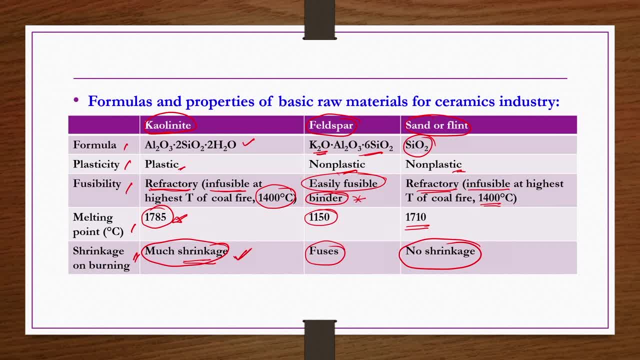 So now you see, one of the material is very much shrinkage, another one is the no shrinkage and third one is the undergoes fusing on burning. So important raw materials, three important materials are having three important characteristics. So proper combination of these materials one has to take as per the requirement of the 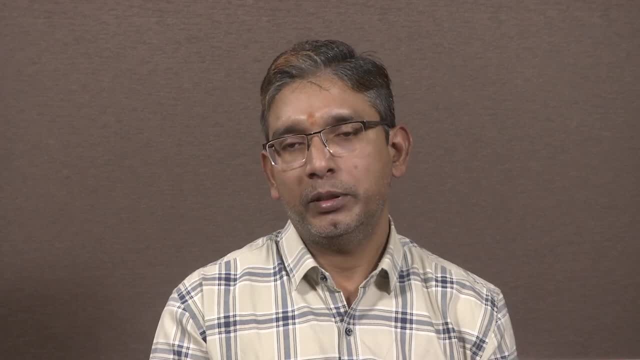 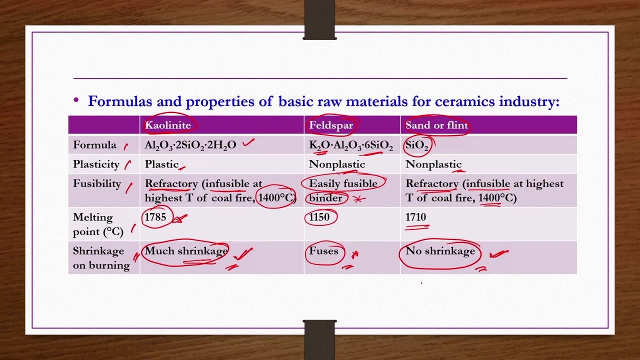 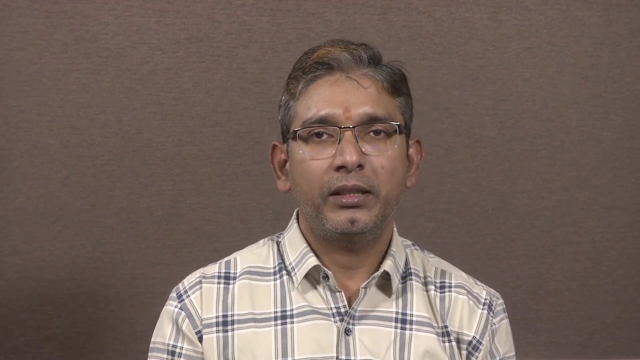 product and then make a required ceramic product. So because of their distinctive characteristics, all of them are very much essential from the ceramic products viewpoint. So that is what we have seen about raw materials. Primarily three important raw materials: clays, feldspar and then sand. 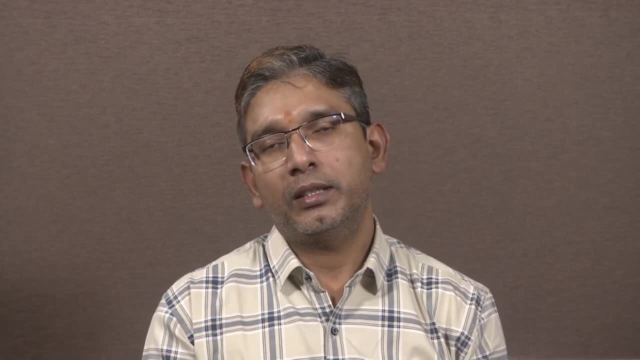 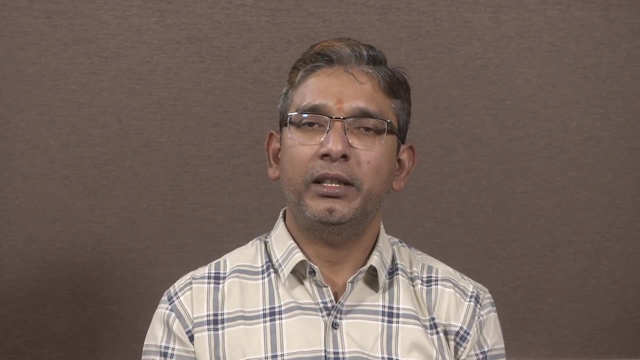 So we have discussed in detail about them, and then we compared properties as well. right, What does it mean by? Does it mean that ceramic industry is having only these three raw materials? No, there are n number of other raw materials are also there. 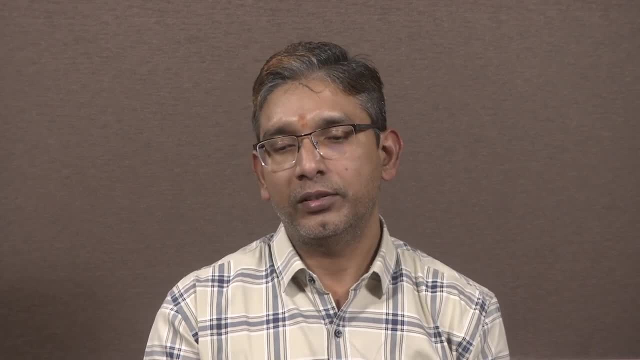 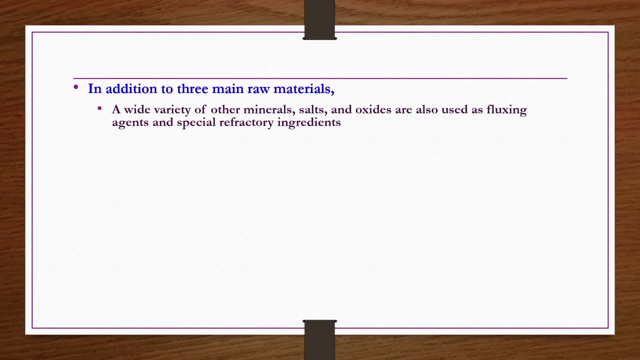 They are also having certain kind of characteristics requirements as well. So those things we are going to discuss now. In addition to three main raw materials, a wide variety of other minerals, salts, oxides are also used as fluxing agents and special refractory ingredients. 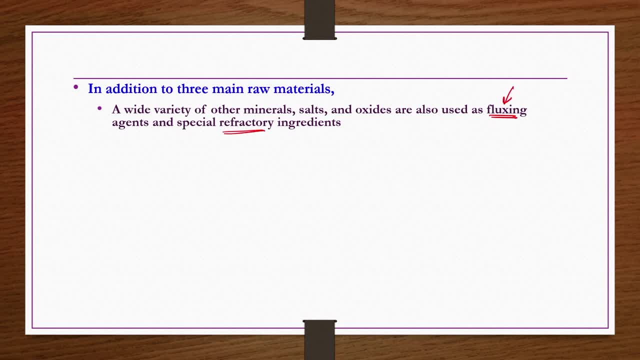 Fluxing agents the purpose. they reduce the reaction temperature. That is the reason you need to have such fluxing agents. And then special refractory ingredients are required because these are infusible even at high temperatures of 1400, 1500 degree centigrade. okay, 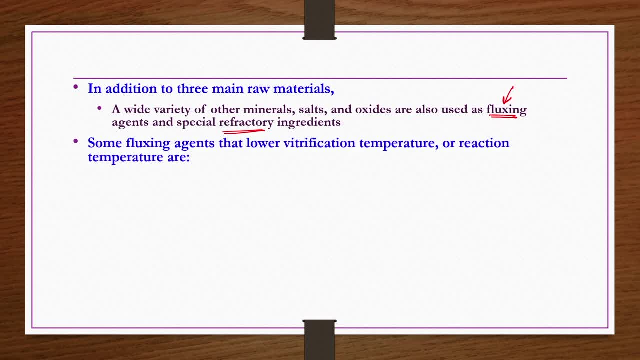 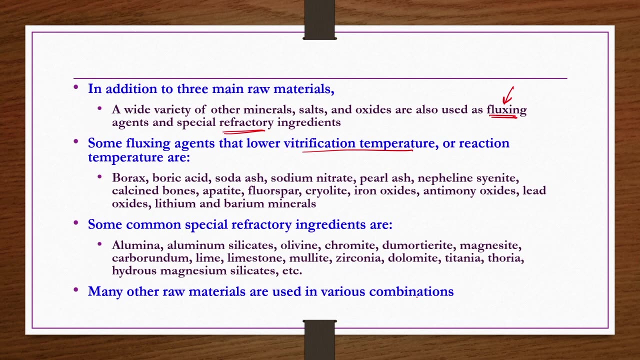 They also provide some kind of vitrification to the product. Some fluxing agents that lower vitrification temperature or reaction temperature are provided here. Likewise some common special refractory ingredients are provided here. Many other raw materials are also used in various combinations as well. 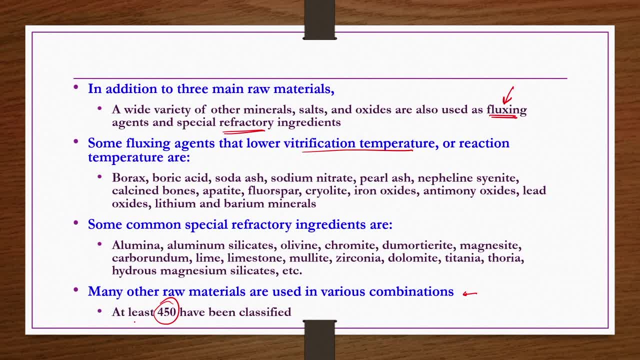 And then at least 450 have been classified as a kind of important raw material from different applications point of view, 450, out of which three are very much essential: clay, feldspar, and then sand or flint. So that is about the raw materials and then their characteristics, importance etc. from. 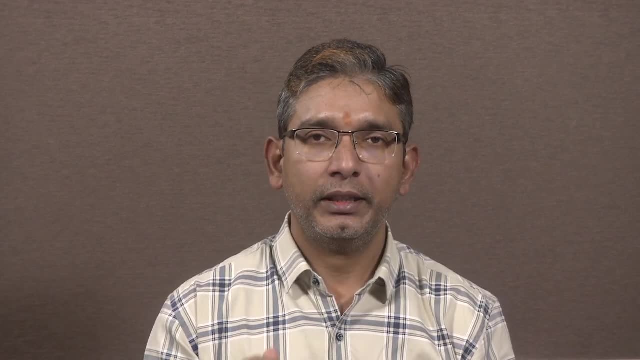 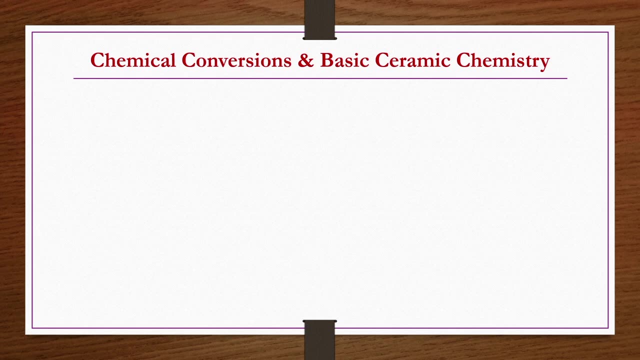 the ceramic industry point of view. Now we are going to see second important topic of the today's lecture, that is, basic ceramic chemistry: Chemical conversions and basic ceramic chemistry. Ceramic products are prepared by combining different amounts of raw materials that we have discussed shaping and heating to firing temperatures. 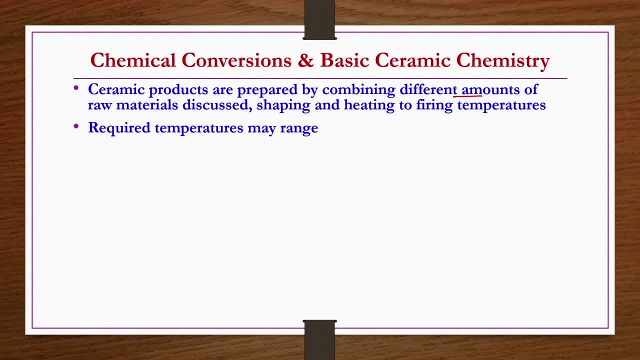 Required temperatures may range. may range from several hundred degree centigrade to several thousand degree centigrade, as well as per the requirement. Let us say, If you wanted to have a over glazed product, then required temperature may be as low as 700 degree centigrade only. 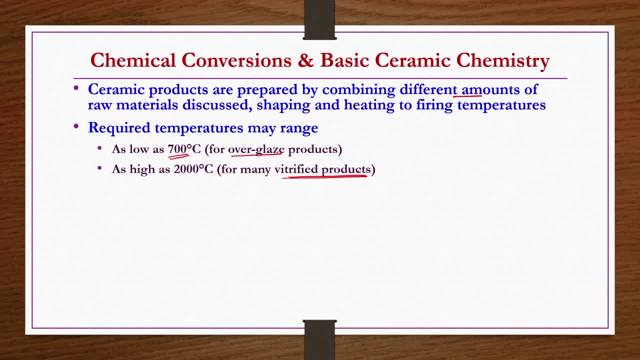 But if you wanted to have many vitrified products, as like glass products, or vitrified ceramic products, etc. So then temperature would be as high as 2000 degree centigrade. Firing at such range of temperatures leads to various reactions which are chemical basis. 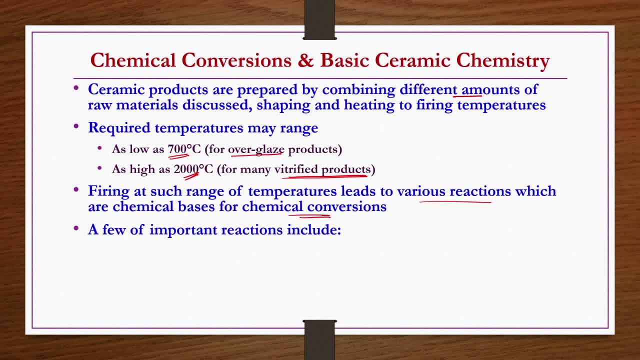 for chemical conversions Right. A few important reactions include dehydration or chemical water smoking at 150 to 650 degree centigrade, Then calcination, for example calcination of calcium carbonate at 600 to 900 degree centigrade, and then oxidation of ferrous iron and organic matter at 350 to 900 degree centigrade. 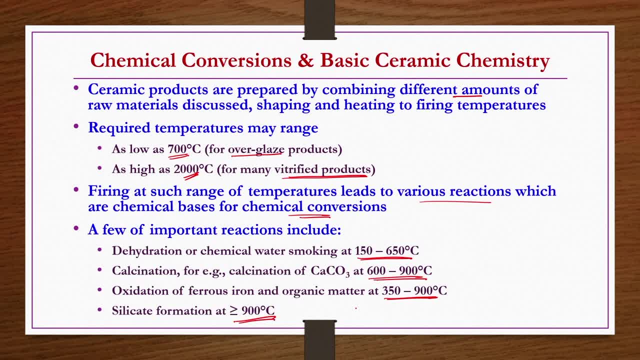 and then silicate formation beyond 900 degree centigrade. Now you see, These are the generalized reaction nature, Not only these reactions. there may be another number of reactions may also be possible- But categorically, if you wanted to present these are the four important reactions that 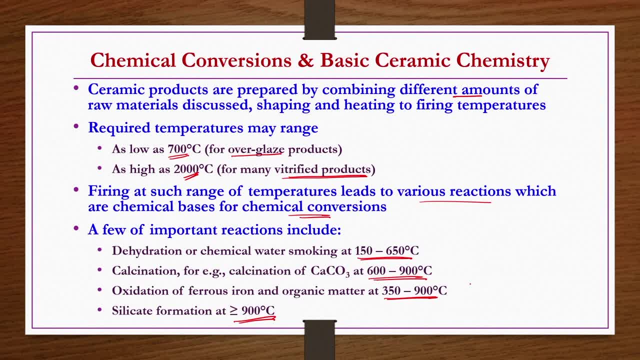 are possible in basic ceramic industry, when the ceramic product is produced. Now they are not like that: individually, step by step, they take place Right. So you can see here, let us say, at 600 degree centigrade dehydration may also take place. 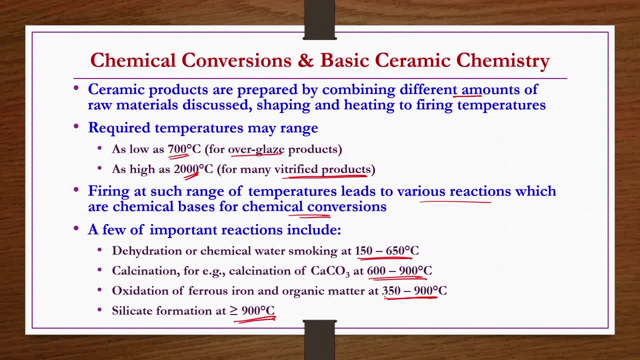 calcination may also take place, and even oxidation of ferrous iron materials may also take place. Right, Okay, So at a given temperature, more than one of these steps may possible, but however, at temperature more than 900 degree centigrade only silicate formation takes place. 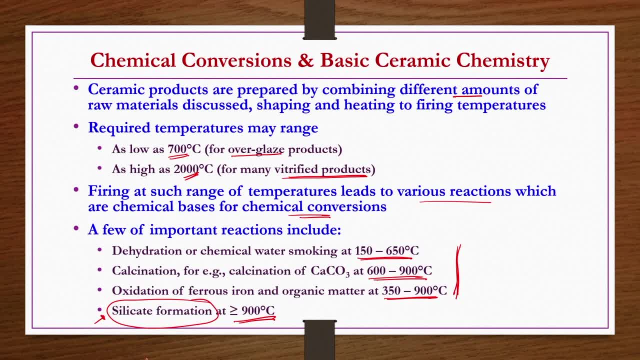 Silicate formation taking place, that means product formation is taking place, Right. And then what you realize here? these reactions, whatever the dehydration, calcination, oxidation reactions, are there simple reactions, Right, There is not much chemistry to understand. But whatever this silicate formation taking place beyond 900 degree centigrade, they are. 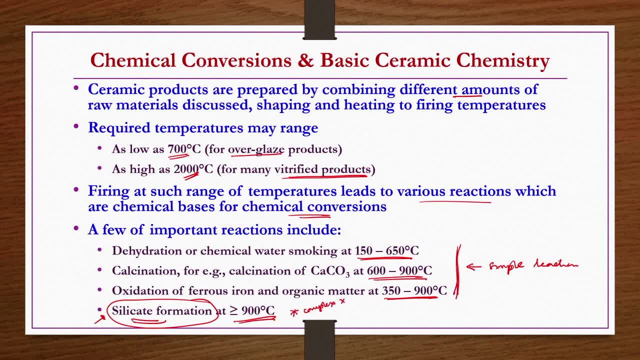 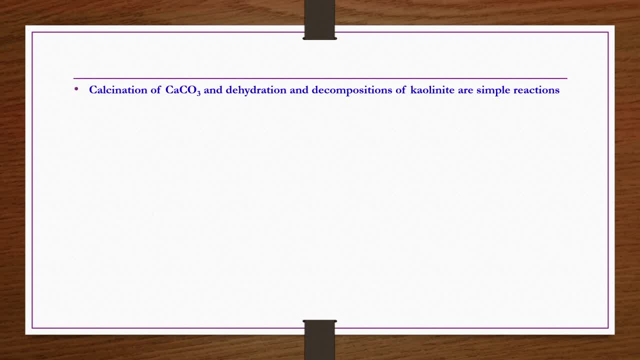 very complex, very complex reactions are there. very difficult to realize them. Okay, So calcination of calcium carbonate and dehydration and decomposition of kaolinite are very simple reactions, but silicate formations are quite complex reactions. These complex reactions obviously change with the applied temperature and constituents of 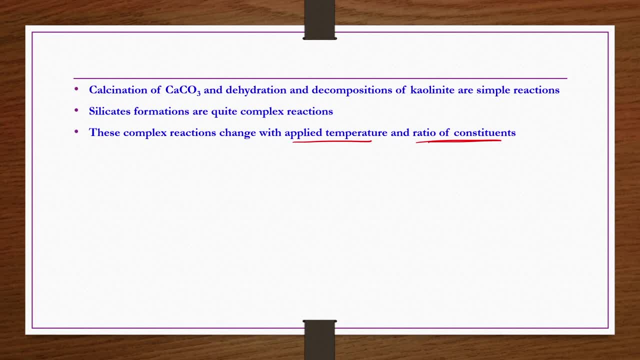 the raw materials. So this has been taken to prepare or to make a given ceramic product. So obviously phase diagram or phase rule in ceramic industries are very important for interpreting empirical observations in ceramic industries and in making predictions for improvements. We are going to see a phase diagram of SiO2Al2O3, then you can realize how much important if 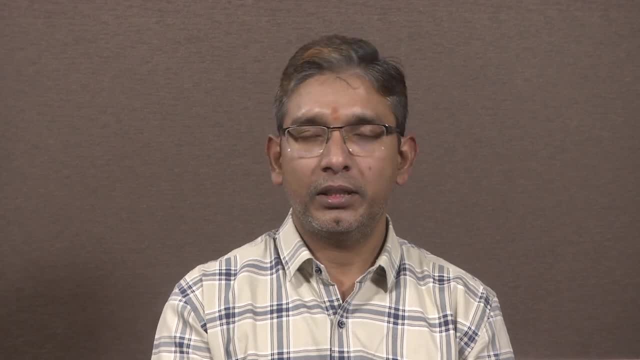 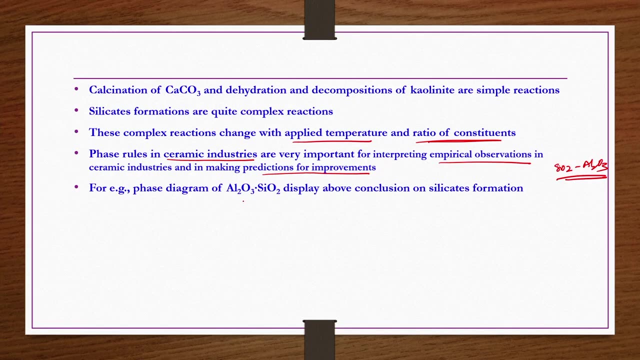 you have the information of phase diagram, Okay, For a given combination of material from the product point of view. Okay, That we are going to see in the next slide. For example, phase diagram of Al2O3SiO2 display above. conclusion on silicate formation. 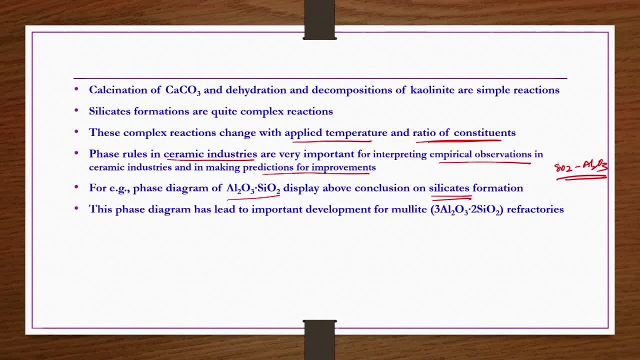 That silicate formation is very complicated reaction. This phase diagram has led to important development of mullite refractories. Right Or the many of the refractories are mullite type refractories which are having 3Al2O32SiO2. 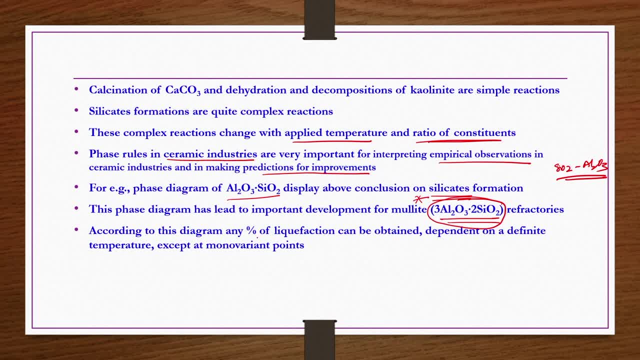 chemical formula. Okay. So according to this phase diagram, any percentage of liquefaction can be obtained. If you have pure SiO2 and then Al2O3,, then it is a different thing, But if you have a combination of these two, any percentage 10 percent to 90 percent. 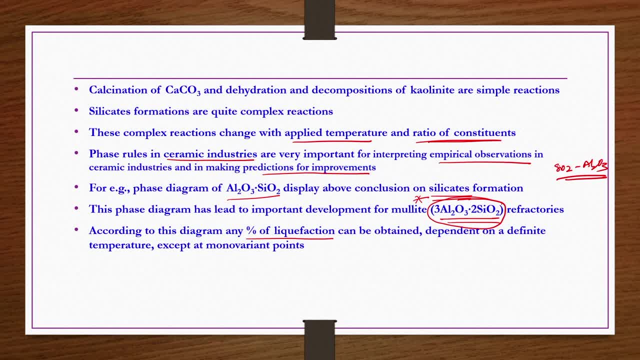 so then you know you can obtain the liquefaction at lower temperature itself, Right? If progressive melting is kept from going too far by controlling rise in temperature, sufficient solid skeletal material will remain to hold hot mass together. Okay, And it shows that mullite is only stable compound of alumina and silica at high temperatures. 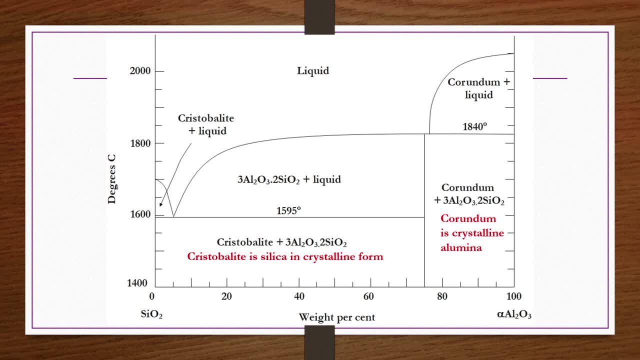 that you see here in this slide. Okay, So now here what we have: a we have a pure silica and then we have a pure alpha alumina. Now, if you have a pure silica, or less than 10 percent alumina mixed with the silica, 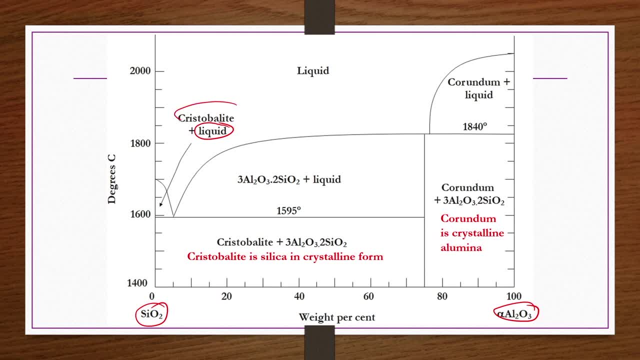 then you know what happens: Liquid and then cristobalite. Cristobalite is nothing but mullite. Okay, So these are the crystalline silica. it is nothing but crystalline form of the silica is known as the cristobalite. that you can get. you know if you operate at the temperature. 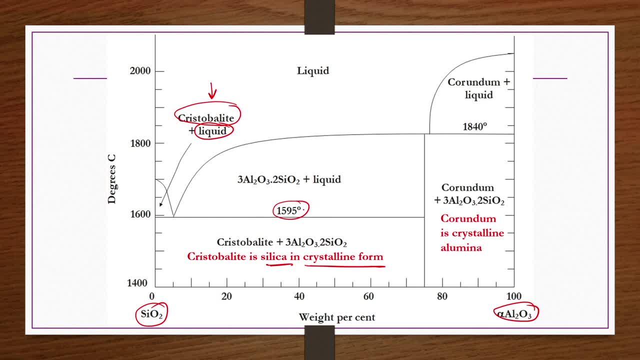 more than 1595 degrees centigrade right, And then if you have almost like pure alumina, that is, you know, only less than 20 percent, 20-25 percent of silica only present, Then you can have a liquid sample plus alumina. 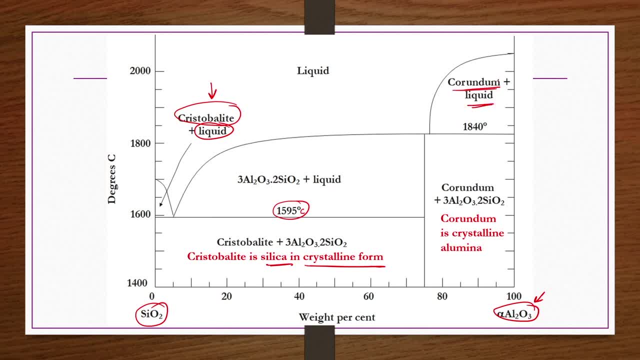 Okay, So this is a liquid sample plus corundrum, which is nothing but crystalline alumina. This corundrum is nothing but the crystalline alumina at temperatures more than 1840 degrees centigrade, Right, But if you have any percentage of these two from you know, let us say 10 to 75 percent. 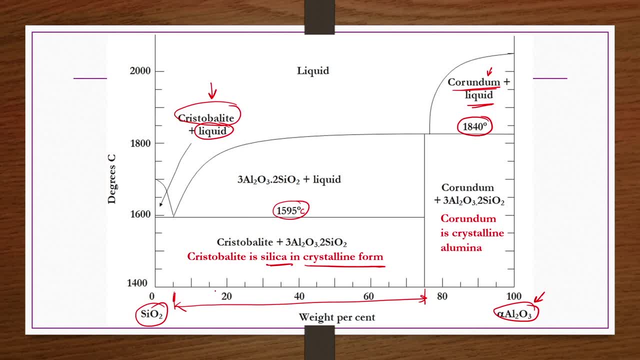 if you take 10 to 75 percent of alumina and silica and then apply the temperature, higher temperatures, what you can see? Okay, Irrespective of the composition, irrespective of the composition in this range, you get mullite. 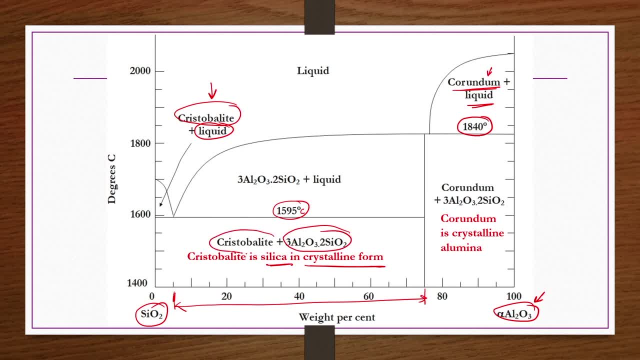 Along with that one, there would also be some cristobalite, which is nothing but crystalline silica. It is possible up to 1595 degrees centigrade, But, however, if you do not want any crystalline silica, you need a liquid sample and then 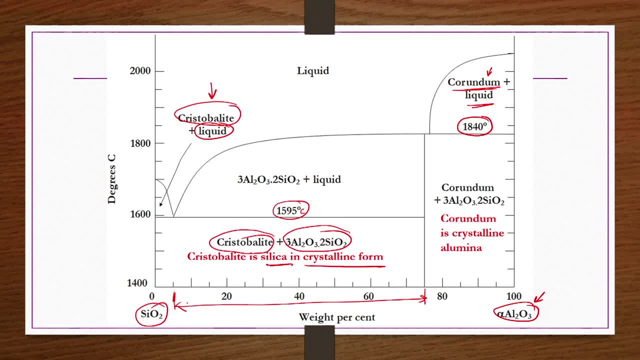 what you do? You further increase the temperature so within the same composition range you can get still mullite you get, and then liquids you get within this envelope where the composition variations are there between 10 to 75 percent of alumina and silica. 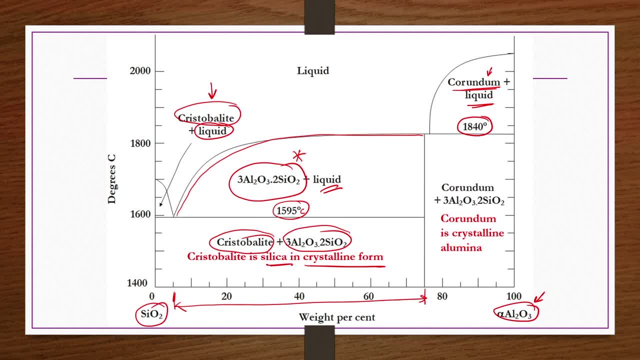 Right. But now here you can see if you have almost like pure alumina, so then corundrum and then mullite. here also you get mullite up to the temperature of 1840 degrees centigrade. But if you go beyond this temperature you do not get mullite. 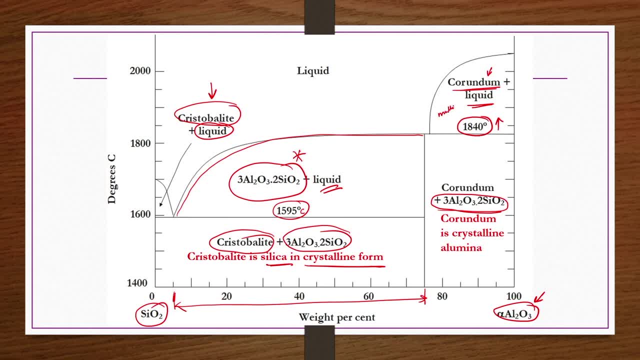 Okay, Okay, So you do not get mullite here, Right Here also for the silica, which is almost pure silica with little alumina, then if you go beyond this temperature of 1595 degrees centigrade, you get liquid as well as the cristobalite. 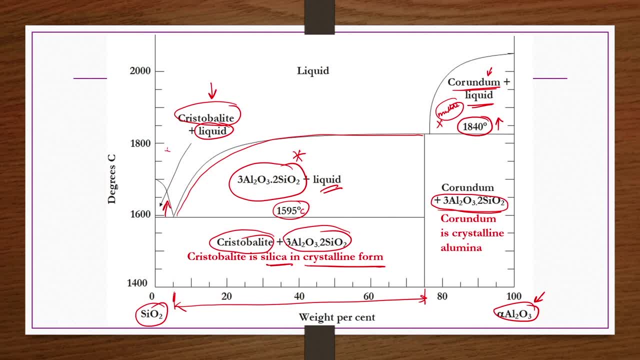 silica, Right, But you do not get any mullite. Mullite has been found to be very good refractory, so if you are targeting that one, so and then what is your source of SiO2 and then Al2O3?? 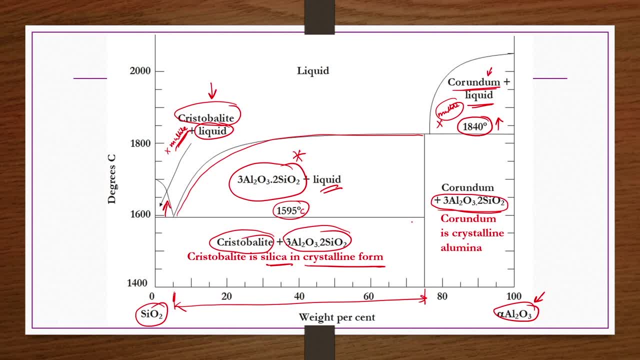 Accordingly, you take a composition and then you make a mixture. so then, definitely you are going to get a mullite, as long as the variation of the composition is between 10 to 75 percent and in temperature it is even at 1400 degrees centigrade also, this formation. 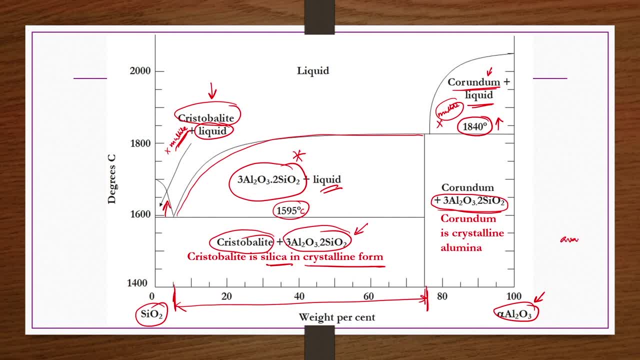 are taking place. So now, availability of these two components and then requirement of the products. what, what do you want to have in the products? You want to have more corundrum in along with the mullite, or you want to have more cristobalite. 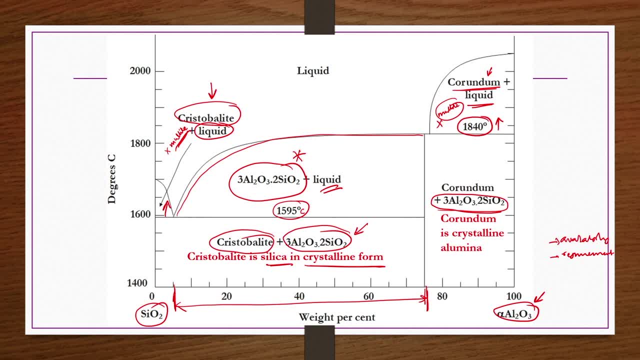 along with the mullite in your final product at higher temperature. so accordingly you can design the composition. accordingly you can design the temperatures: application temperature. Okay, So now you can see how much essential to understand phase diagram If you have a phase diagram so you can get so much information. 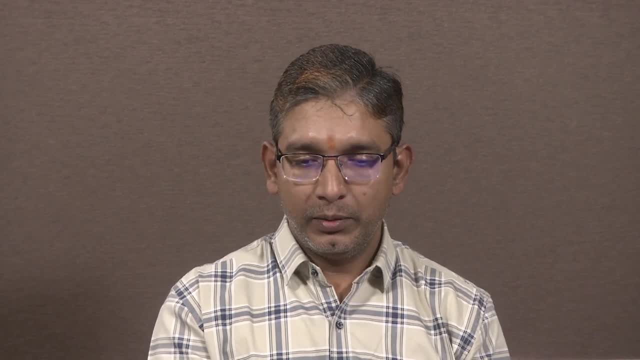 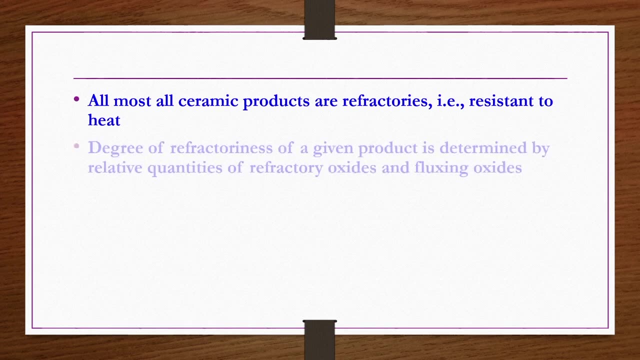 So from the product point of view- let us say mullite is one of the example here- Almost all ceramic products are refractories, that is, resistant to heat. degree of refractoriness of a given product is determined by the relative quantities of refractory oxides and fluxing. 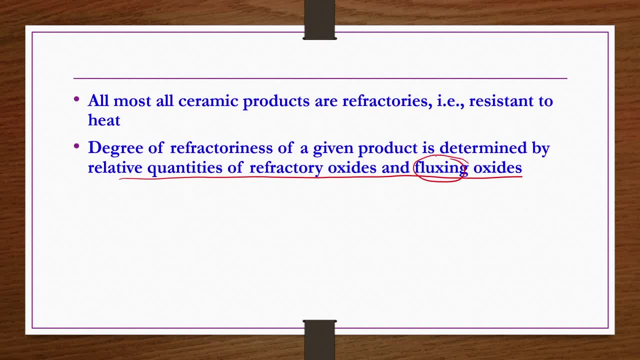 oxide, Fluxing oxide we have seen. so fluxing oxide they reduce the reaction temperature or vitrification temperature, whereas the refractory oxides they provide required thermal resistance or thermal stability. Important refractory fluxes are given here, but there are some less commonly used to fluxes. 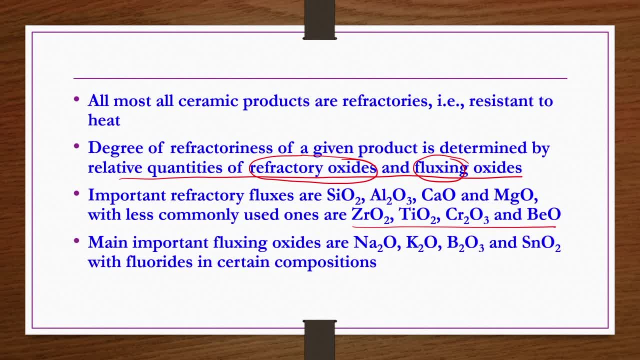 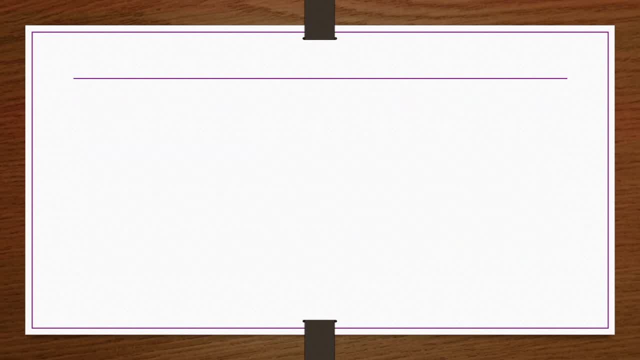 refractory fluxes are also there. they are here given here Main important fluxing oxides are these things with fluorides in certain compositions are also possible. So now what we understand until now in ceramic products, clay such as kaolinite, mostly not. 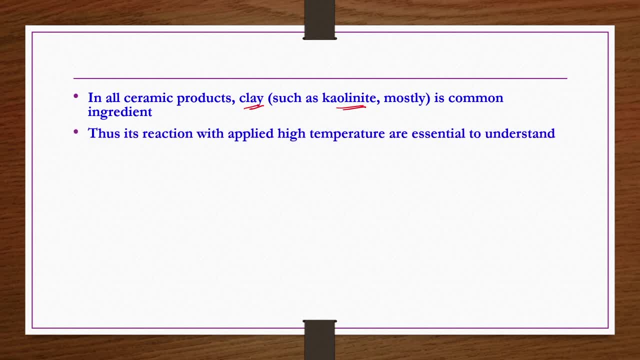 the only one is a very common ingredient And then thus its reaction with applied high temperature are essential to understand. So at 600 to 650 degree centigrade the applied energy drives off the water of hydration, that is, dehydration reaction etc. takes place. 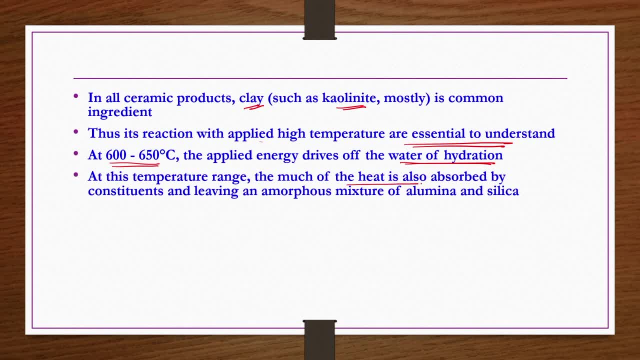 Further at this temperature what happens? much of the heat is also absorbed by the constituents and leaving an amorphous mixture of alumina and silica, as per the reaction. let us say you have kaolinite And then supply the temperature of 600 to 650 degree centigrade, then you can get amorphous. 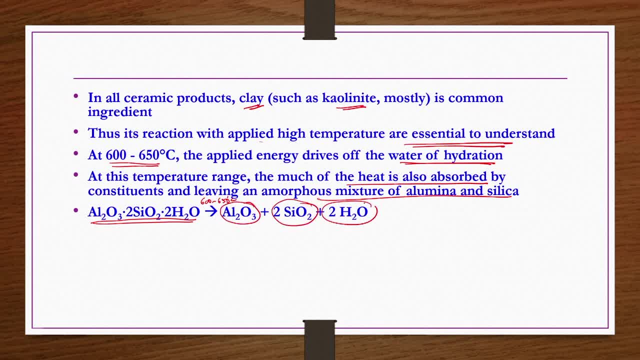 alumina, amorphous silica, along with the water vapor. So not only the dehydration taking place but also getting the amorphous constituents of the mixture, individual components of the mixture you get in the amorphous form. that is, alumina and silica you are getting in amorphous form. that is possible reaction. 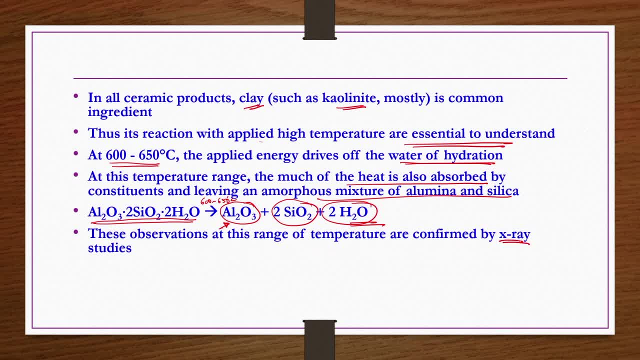 These observation at this range of temperature. So the high temperature are confirmed by the x-ray studies. Actually, these are taking place in high temperature furnaces etc. all those you know, refractories, etc. Then how to realize what is happening, what components are forming, etc. 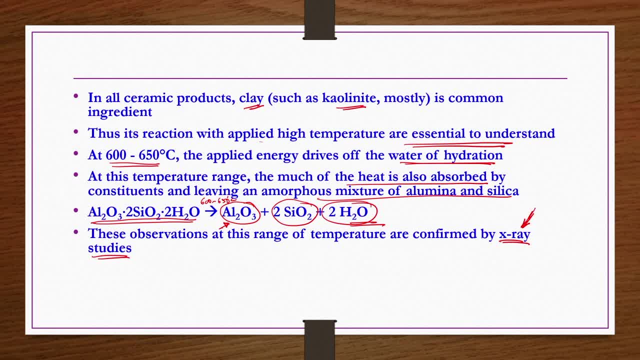 So for those kind of solid state physics point of view, x-ray diffraction is one of the easily available tool to confirm the product formation. What are the products are being formed? okay, A large portion of alumina can also be extracted with hydrochloric acid. 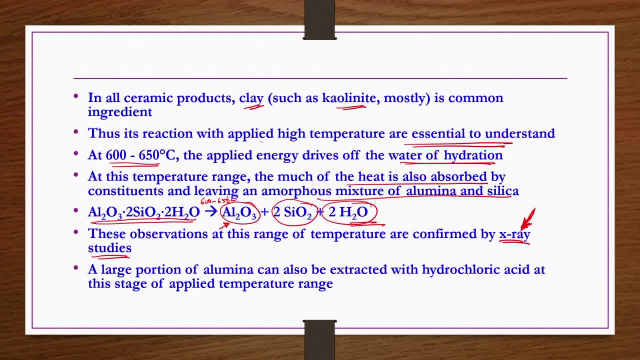 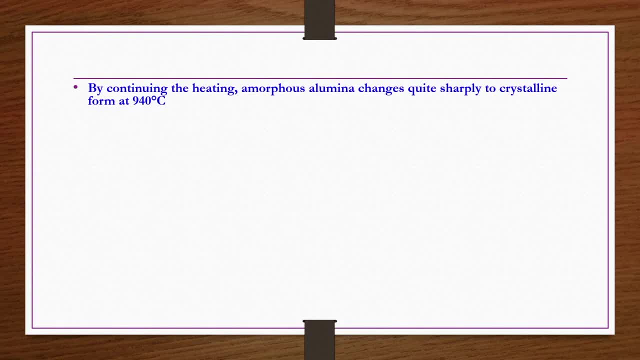 Hydrochloric acid at this stage of applied temperature range as well. Now what happens if you keep on increasing the temperature right? By continuing the heating, amorphous alumina changes quite sharply to crystalline form at 940 degree centigrade by forming corundrum. corundrum is nothing but crystalline alumina. 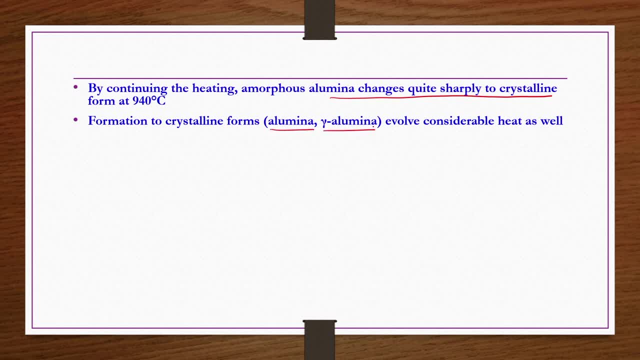 Formation to crystalline forms of alumina or gamma. alumina evolve considerable heat as well. So at starting range of 1000 degree centigrade you are gradually increasing temperature, so 600 to 650 degree centigrade. what happens? 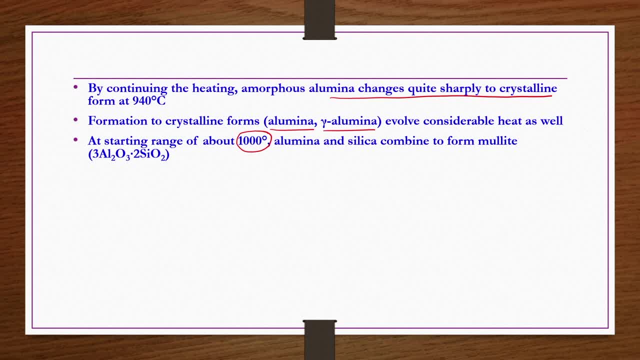 Mostly dehydration takes place, plus formation of the amorphous alumina and silica formation may also take place, as per the phase diagram. those things we have seen. But if you further increase the temperature to 940 degree centigrade, etc. what you are getting? 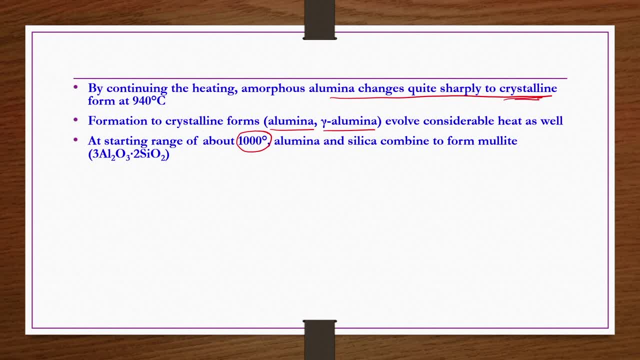 You are getting in a crystalline form of alumina. If you further increase the temperature to 1000 degree centigrade, what happens? Dehydration takes place. If you further increase the temperature to 1000 degree centigrade, what happens? 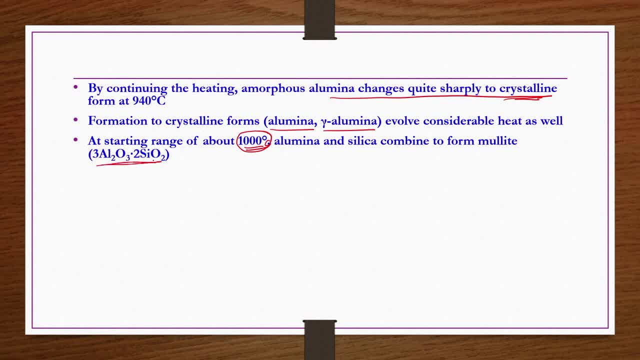 Alumina and silica combine to form molybdite, so this is very essential. this is the one of the base refractory that is available At further higher temperature. remaining silica is converted into crystalline cristobalite. Cristobalite is nothing but crystalline silica, so thus, overall fundamental reaction in heating. 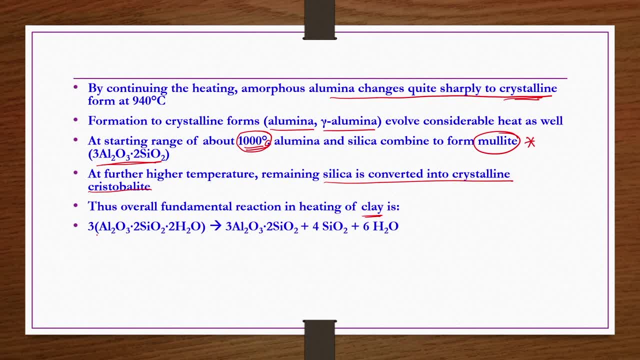 of clay. is this one Like cavalanite? 3 moles of cavalanite. 3 moles of cavalanite. If you react, you get 3 moles of molybdite and then 4 moles of silica and 6 moles of. 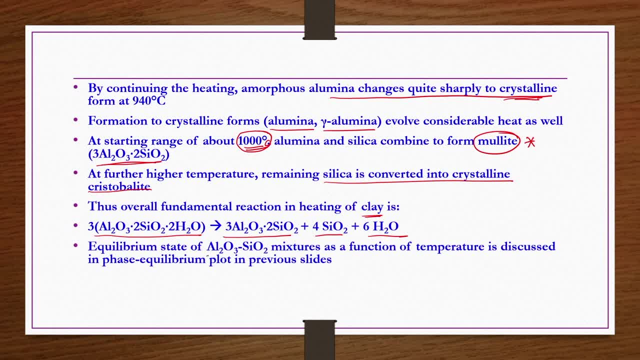 water vapor. Equilibrium state of alumina and silica mixtures as function of temperature is discussed in phase diagram anyway. Presence of fluxes tends to lower the temperature of formation of molybdite and speeds of the approach to equilibrium. so that is the importance of this: fluxing agents. 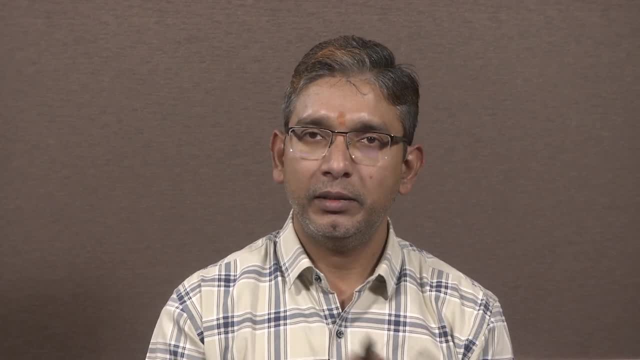 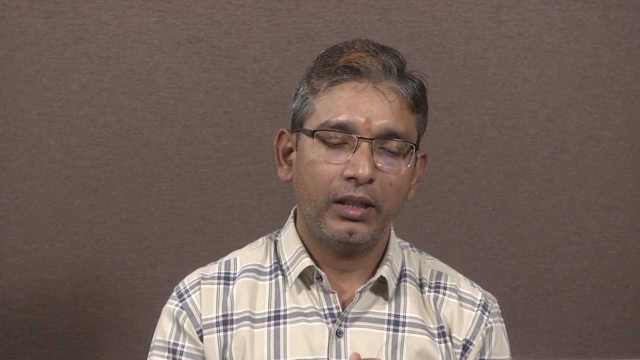 Now we have seen 3 moles of molybdite. So we have seen that 3 are main important raw materials: clay, feldspar and sand or flint, etcetera. So but we also realize there are many other raw materials are also there. they may be. 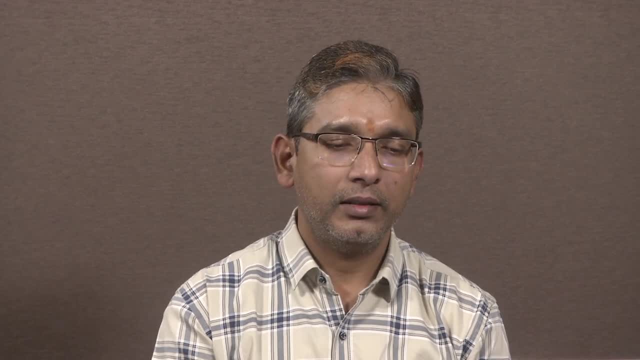 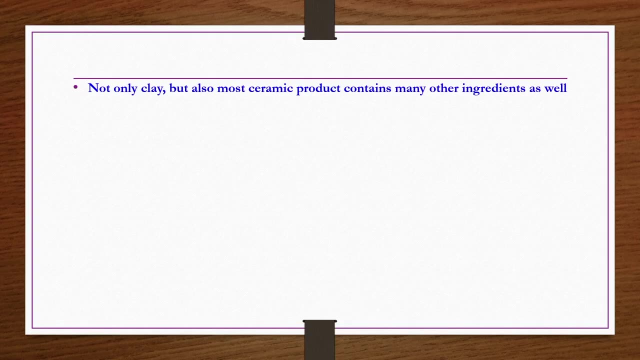 in minor quantities. So obviously not only the reaction that we have discussed in the previous slide, many other reactions may also possible. Not only clay, but also most ceramic product contains many other ingredients as well, so thus there will be many other reactions involved in the process. 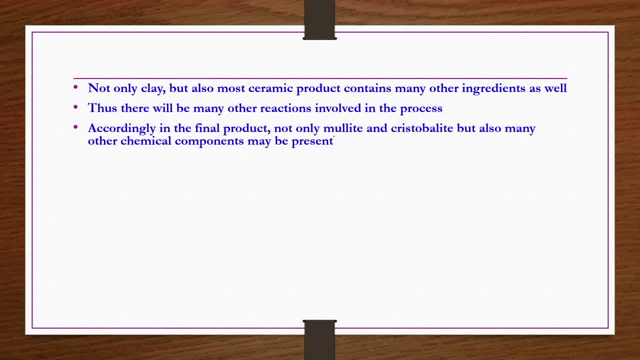 And accordingly in the final product. not only molybdite cristobalite but also many other chemical components may also be present, obviously. For example, various silicates and the aluminates of calcium magnesium and possibly alkali metals may also be present in the final product, but alkali portion of feldspar and most of 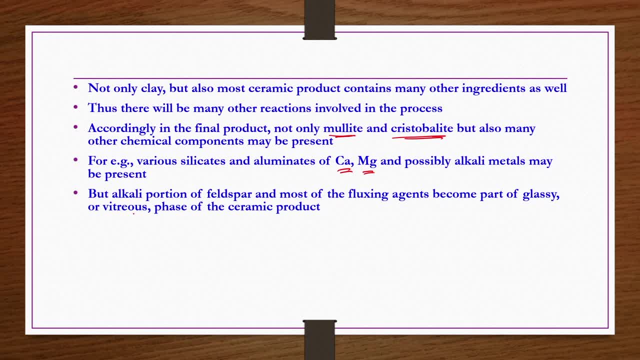 the fluxing agents become part of glassy or vitreous phase of the ceramic product. Okay, In other words, during heating all ceramic products undergo a certain amount of vitrification or glass formation. So what do you understand? Ceramic products you can see now as a kind of some kind of crystalline material plus. 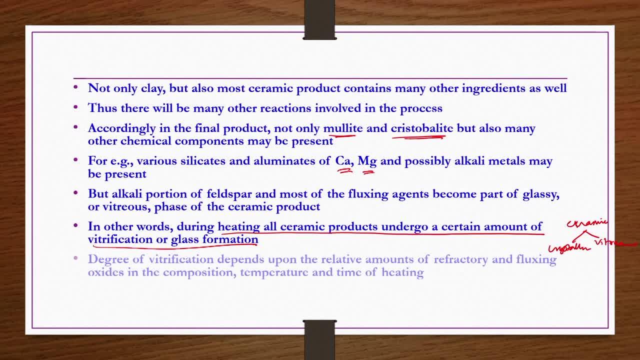 some kind of vitreous nature. Okay, So thus, degree of vitrification depends upon the relative amounts of refractory and then fluxing oxides in the composition, and then temperature and time of heating. Thus, any ceramic product may be said to consist of a vitreous matrix plus crystals, of which 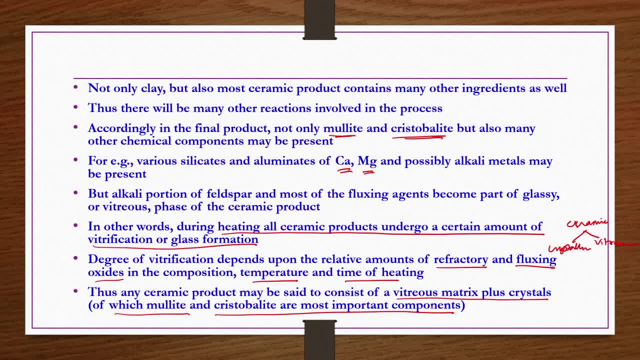 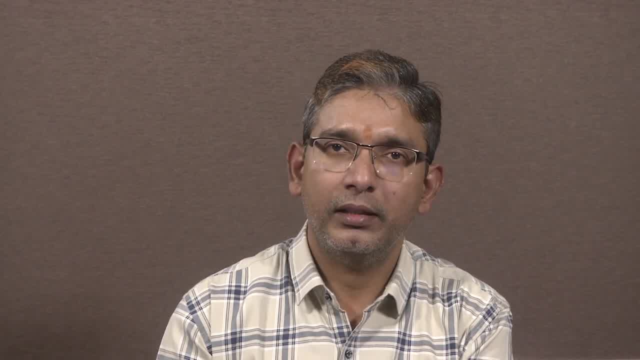 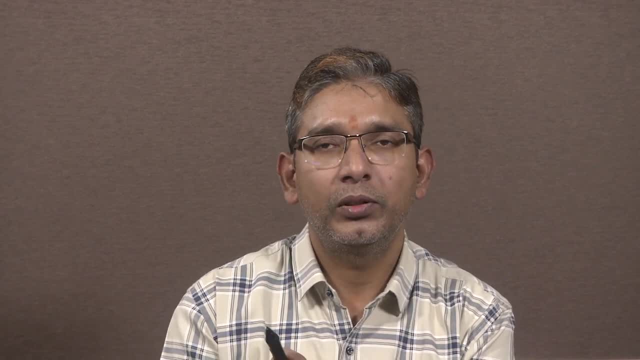 molybdite and cristobalite are most important components. Okay, Now we have already realized that any ceramic product may be said as a kind of vitreous matrix with crystals. So now, based on the degree of vitrification, we try to do a classification right. 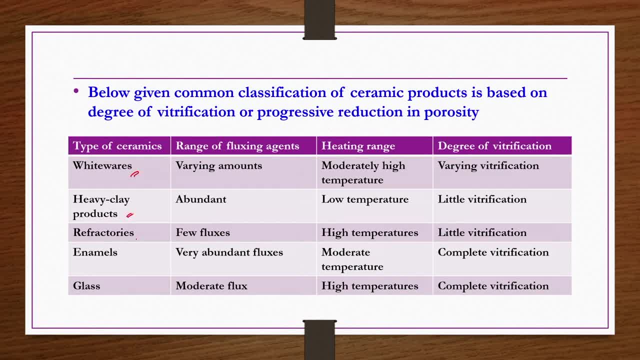 Then what we have- White wears, High clay products, refractories, enamels, glass- we are taking under the types of ceramics- Then what are the corresponding fluxing agents, heating range and degree of vitrification we have here. If you have white wears, so then fluxing agents, range varying amounts have, and then heating. 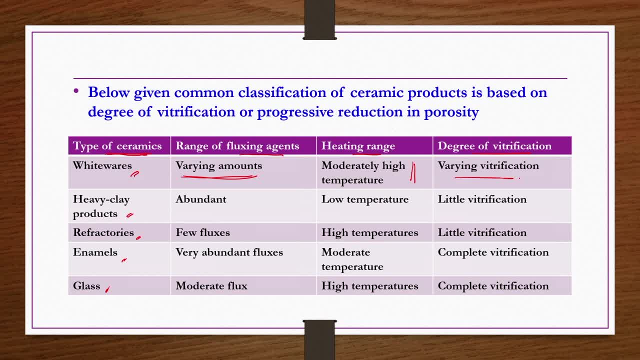 range may be moderately high temperature. So varying degree of vitrification is possible because varying amounts of fluxing agents you are taking And then also the applied temperature is moderately high temperature, whereas in heavy clay products fluxing agents are present in abundant but despite of that one vitrification is not high.